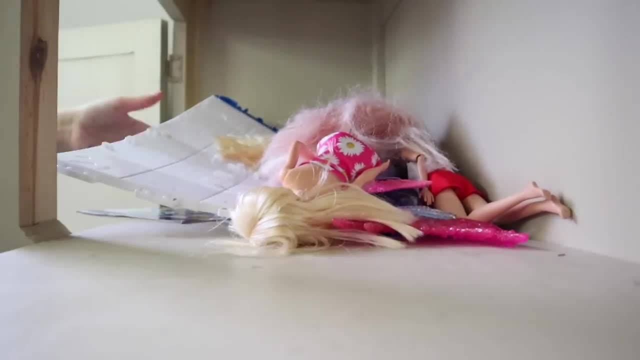 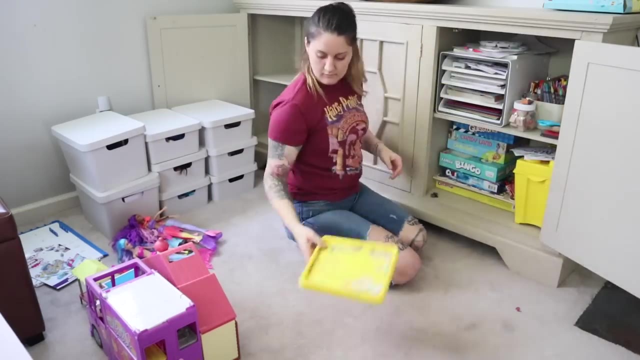 we are going to use the kitchen sink for a tiny little while. You can't really see it without the sink, but it's just a really quick wash that can be done and we're going to do some cleaning up here. So we have a really simple kitchen sink here. 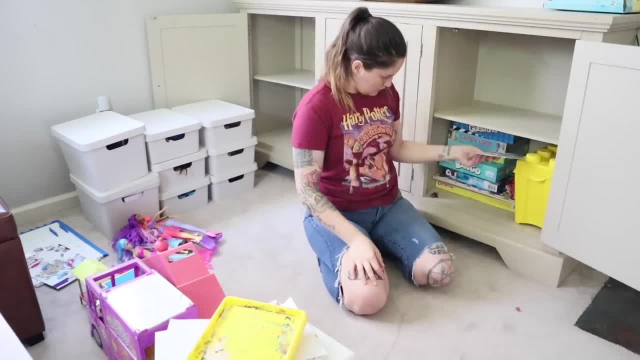 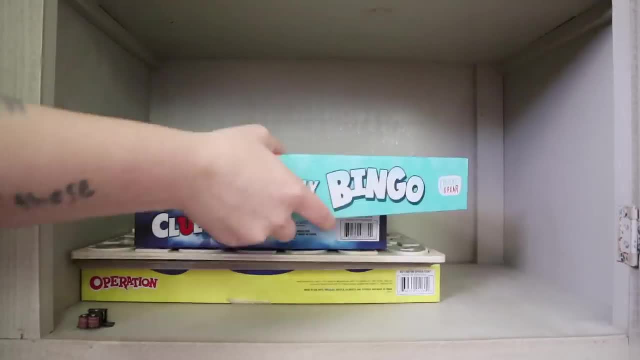 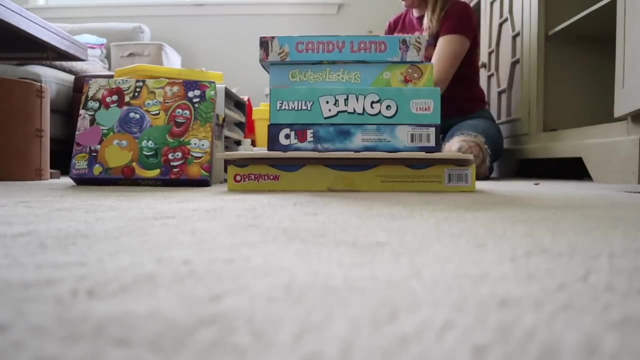 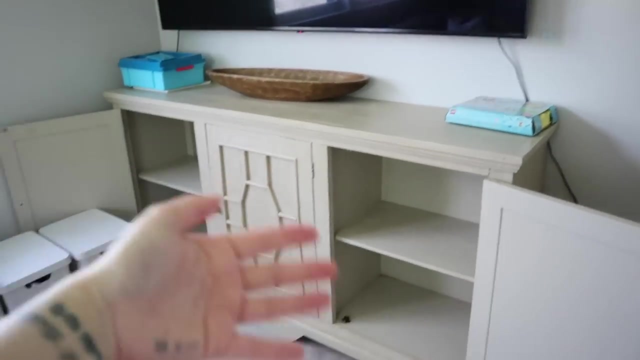 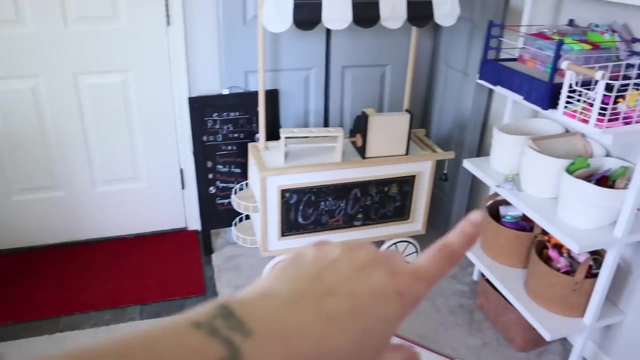 We're going to remove everything from this van. We're going to use our jewelry box, okay, so i just cleared out our media console under the tv, which is where we keep, like i guess, most of the toys, and my original plan was to clear this out and then take all of this. 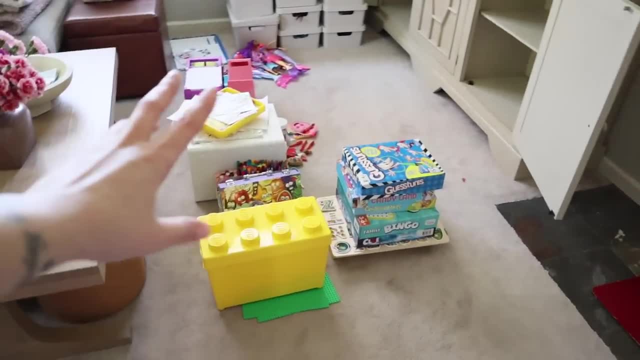 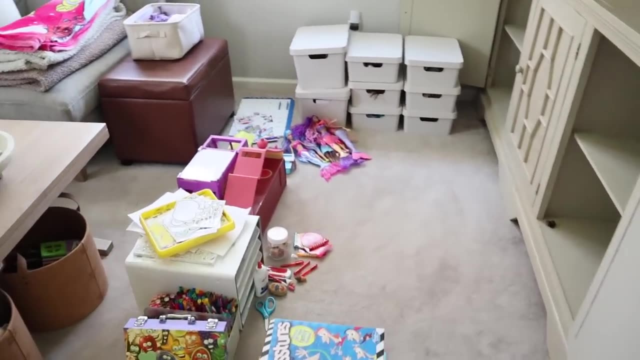 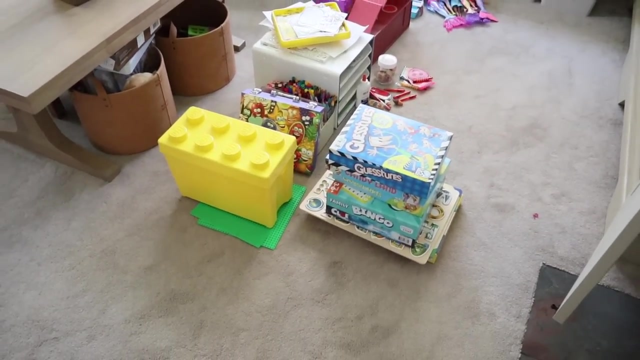 stuff like all the toys in the whole room, to just bring them into one place, cover the floor space with them and then declutter that way. but for one, i'm already feeling overwhelmed with this. like this is a lot. i guess i just forgot how much was in there. but also we don't really have much more. 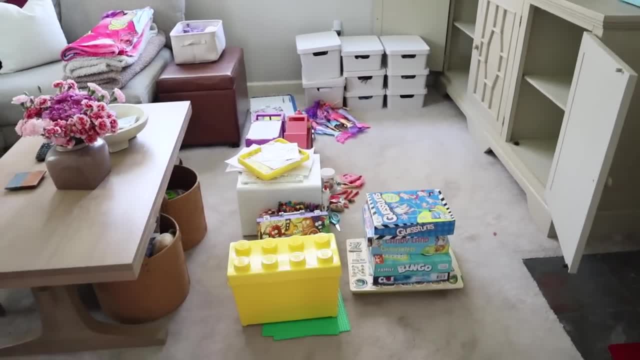 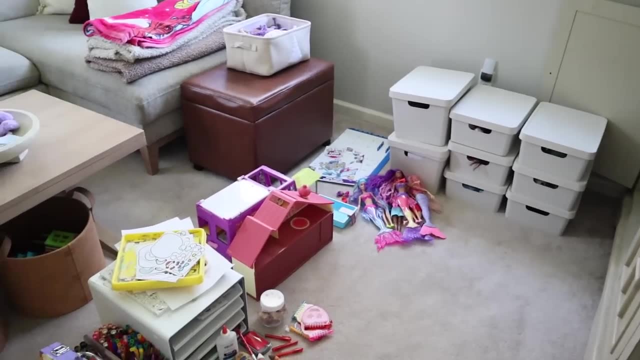 floor space to be able to do that, and i don't want to overwhelm myself to the point where i just like won't do it at all. so we're gonna pivot a little bit, we're gonna take it space by space and then, if i feel like i need to, i'll pull it all out again and do it all at once. but there's just like 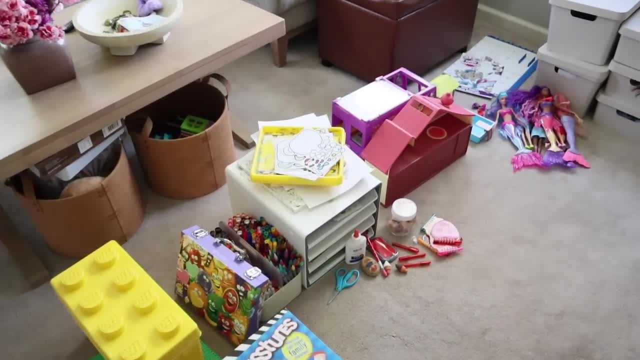 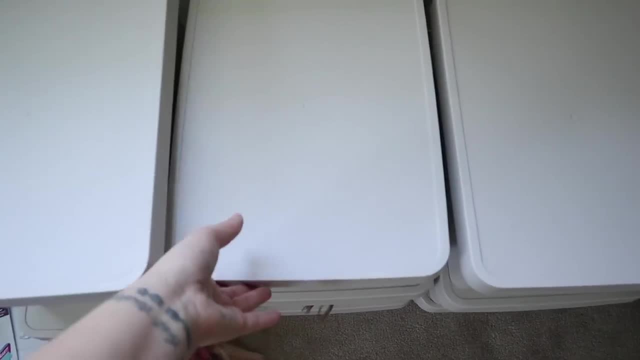 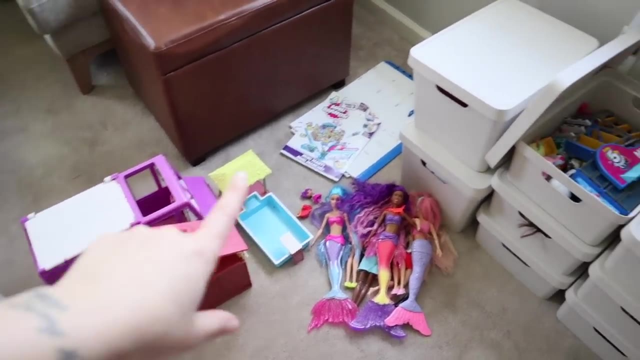 so much other stuff that i'm just gonna go in categories so i kind of have it sorted out here right now. all of these are bins of toys that the girls play with, a lot like their barbies and just like little toys, things like that. these are bigger activities that go with these toys. 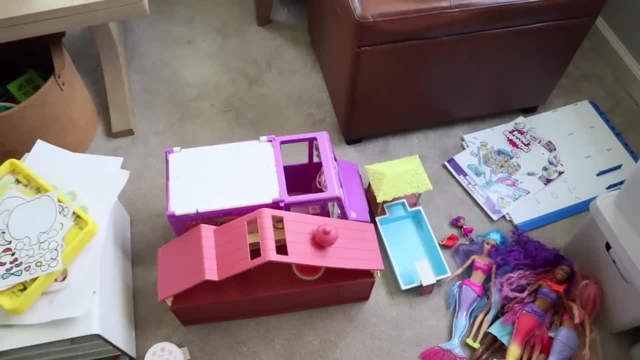 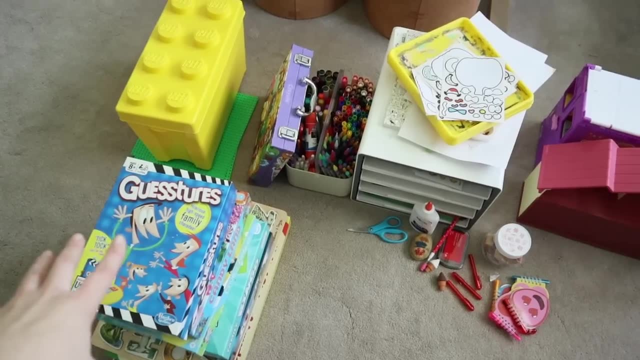 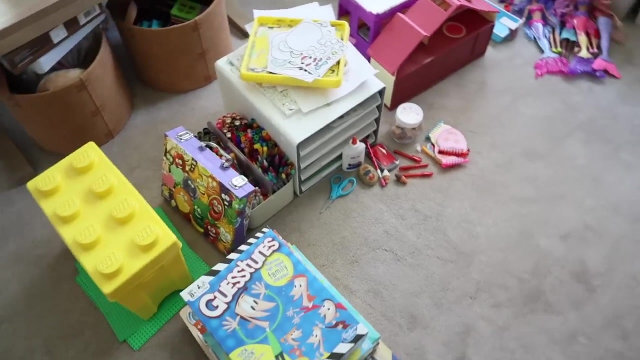 like the bluey house and their taco truck for their barbies, and then i have all the art supplies here and board games and things. so i think i'm going to start over here because it feels like the least overwhelming category and it'll be the fastest to declutter, which will give me that like. 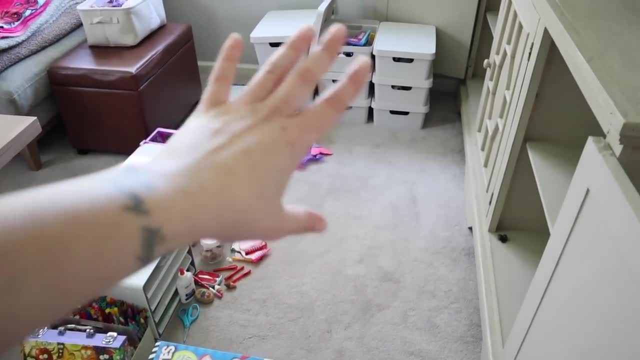 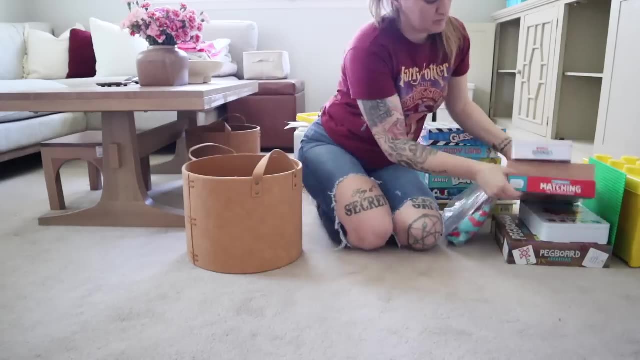 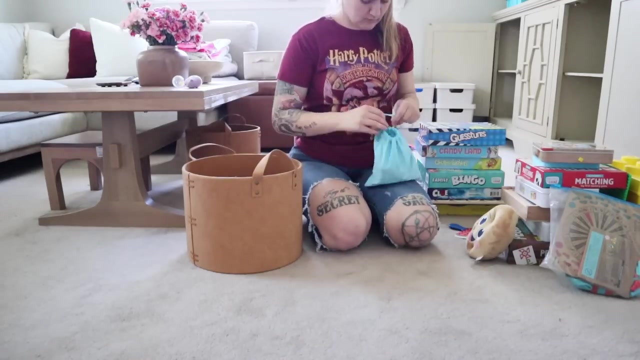 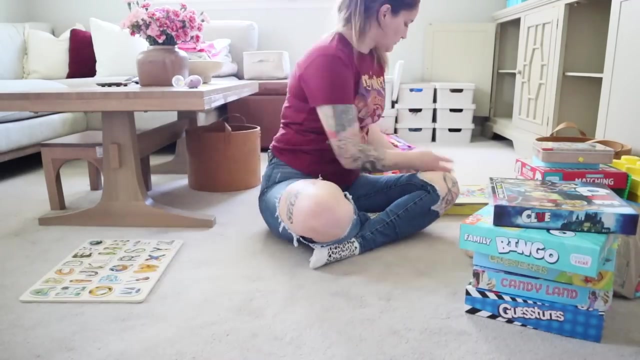 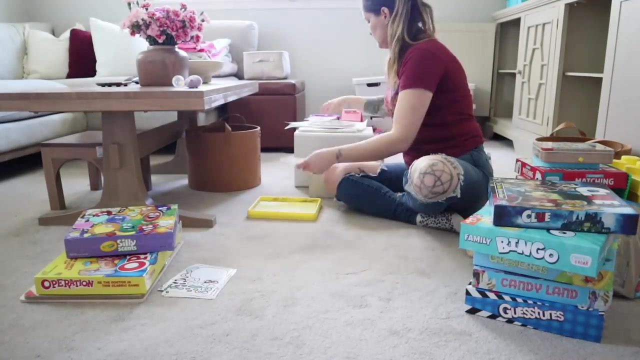 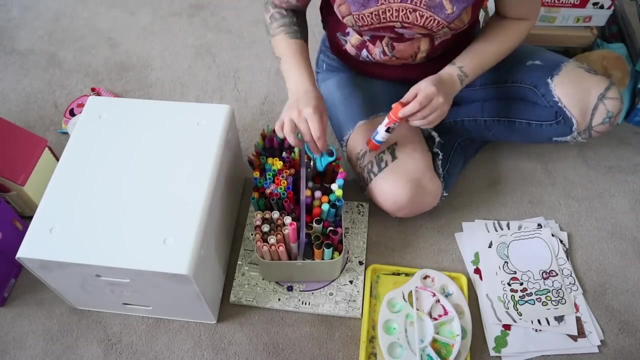 instant gratification and motivation to go through that whole hot mess over there. if i can't be with you, i'd rather be by myself. i know i can't lie, i don't want anybody else. those happy days that we once knew, so long ago, they still. 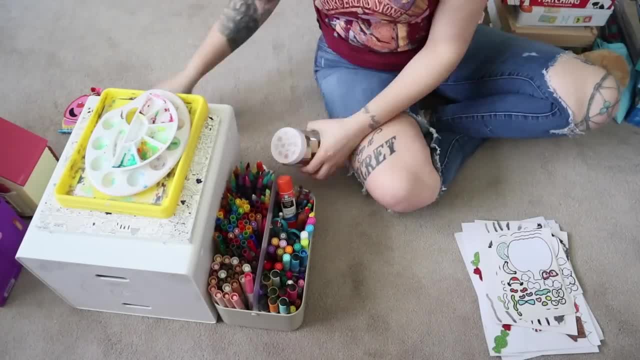 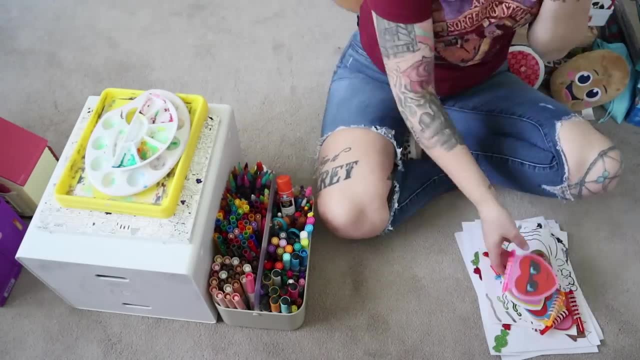 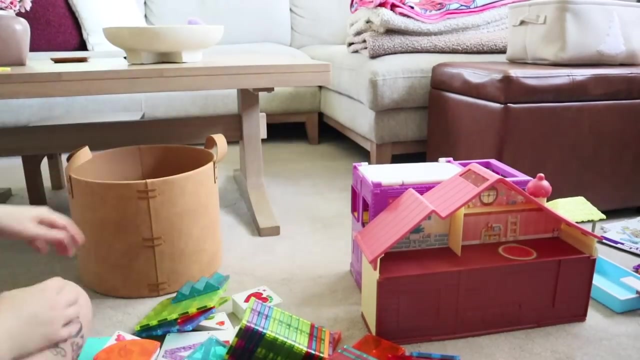 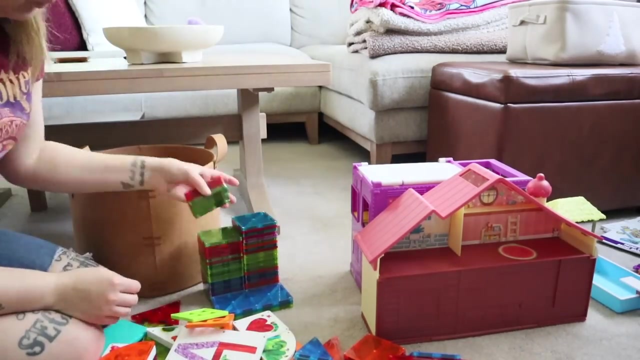 make me blue. i want you right, right, right now. if i could show you somehow how much you mean to me, if you could only see baby. you know, i don't want anybody else, no one but you. you make me feel the way i do. all that i want is to have you to myself. 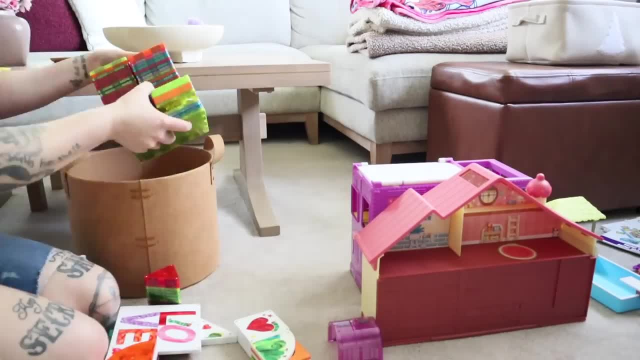 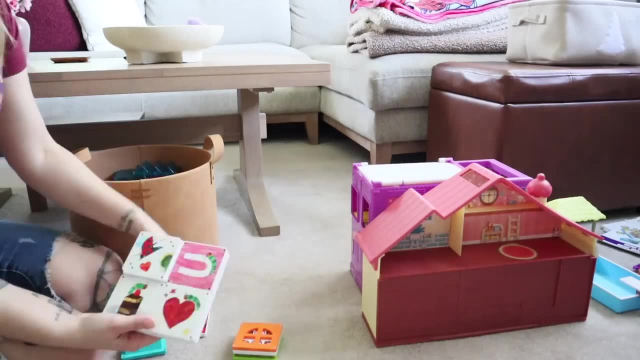 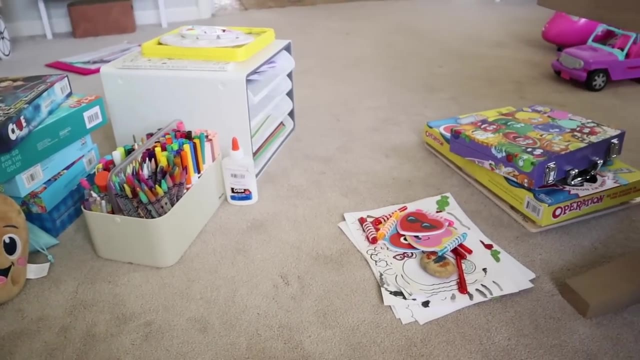 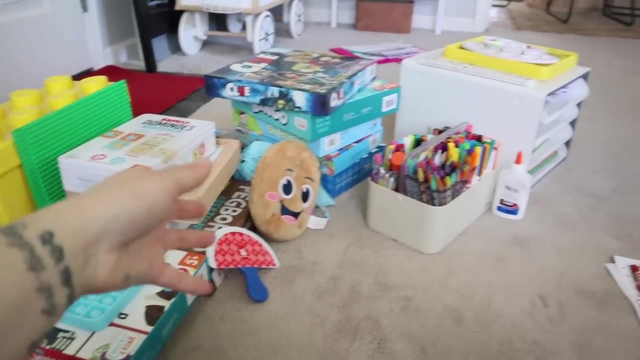 you make me feel the way i do. no one but you. you make me feel the way i do the way i do. maybe i should have started with a different category, because here's our declutter pile and here's the keep pile and clearly they are very uneven. these are just a few things to throw in the trash, but 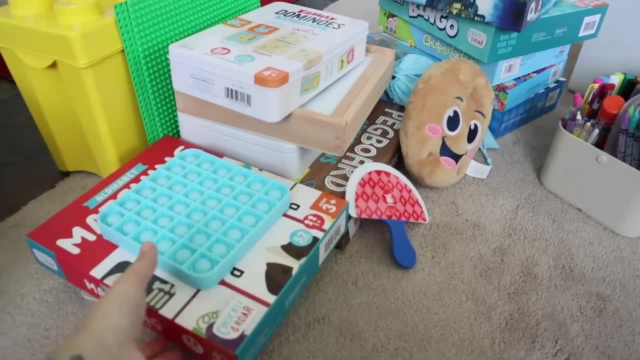 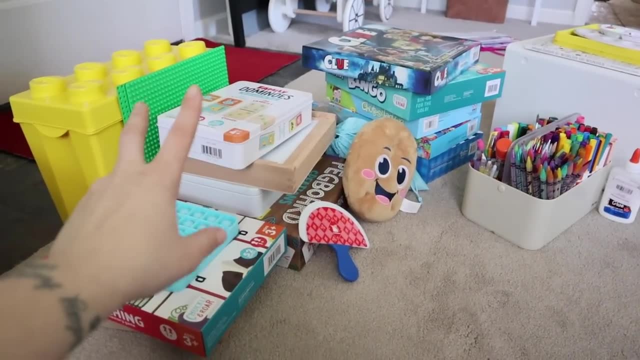 yeah, maybe i should have started with a different category more. but maybe we should have started with a different category because these are all of our board games and family activities, learning activities. it's our play lot with these all the time, so there wasn't much to declutter here. i really 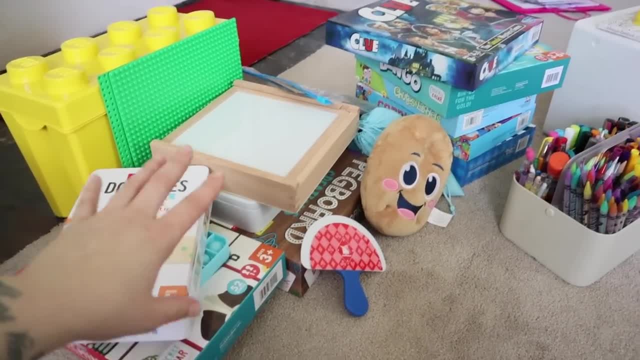 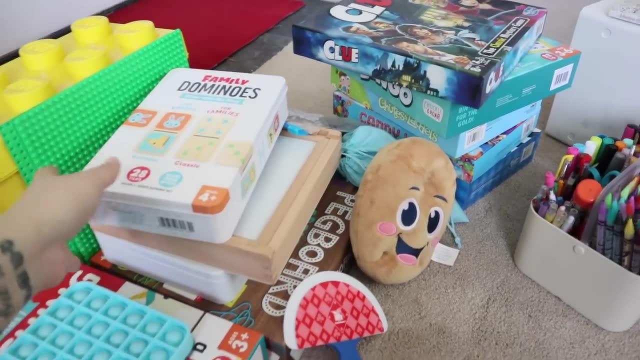 didn't needed to stop climate. they're access to learning activities and PSA like decrease the amount of family activities. we do so as long as we're using and I don't see any points decluttering them across just because something might have given it a hold out for me. 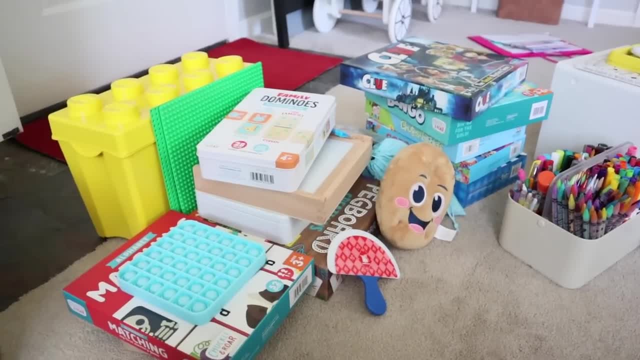 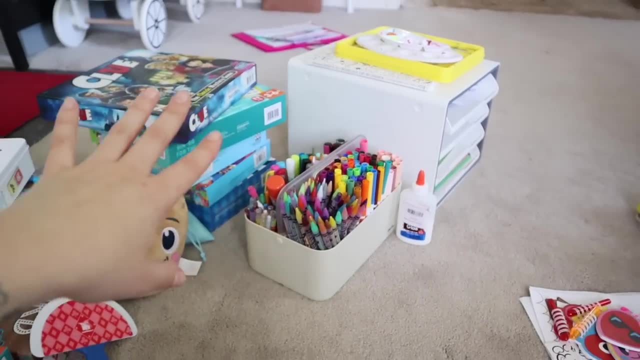 dem, because I mean there is a lot, but we use them and we enjoy the variety, so these are all going to stay. also, if you've been around for a while, you know the art supplies are non-negotiable. both of our kids are so creative. they use those all the time. they're constantly going through them. so I'm 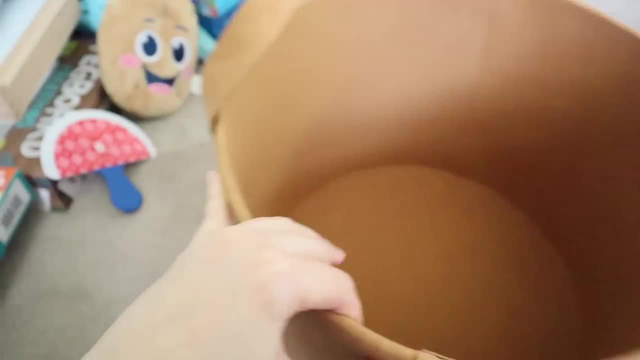 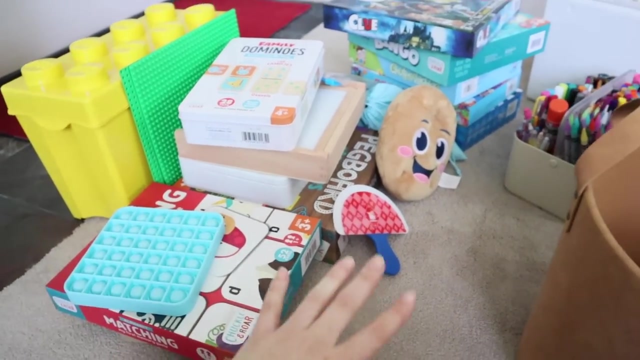 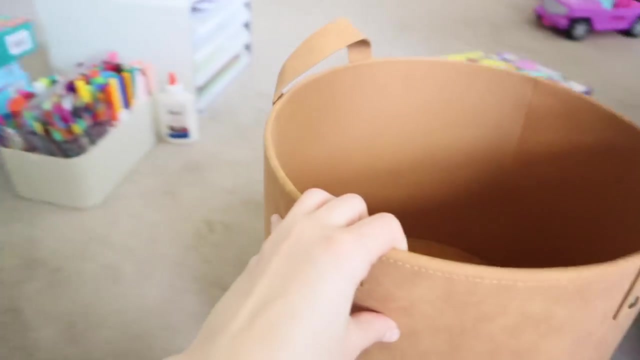 going to repack this bin here with all the smaller toys and things that the girls can play with by themselves, and then all of the games that require like two or more people. I think I'm going to end up putting back in the cabinet, but I do want to keep some things out for them because I find when 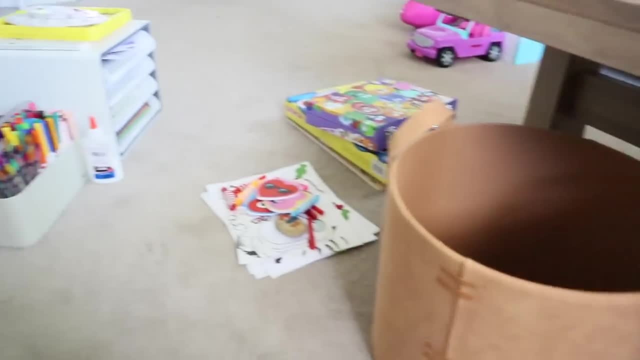 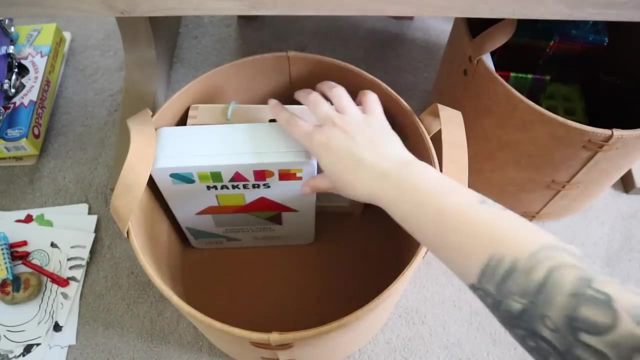 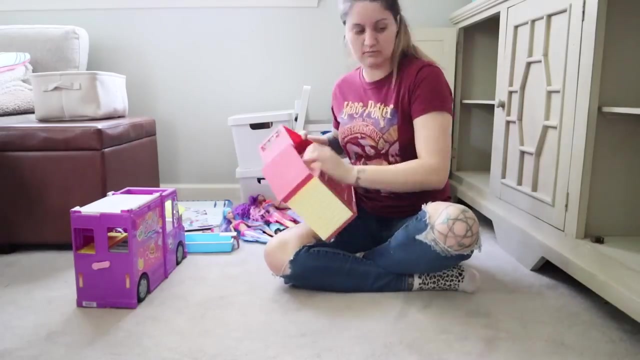 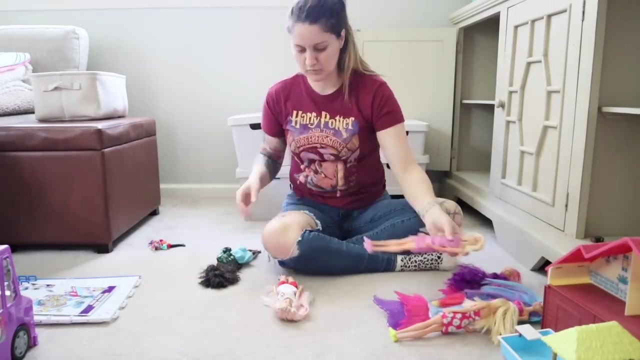 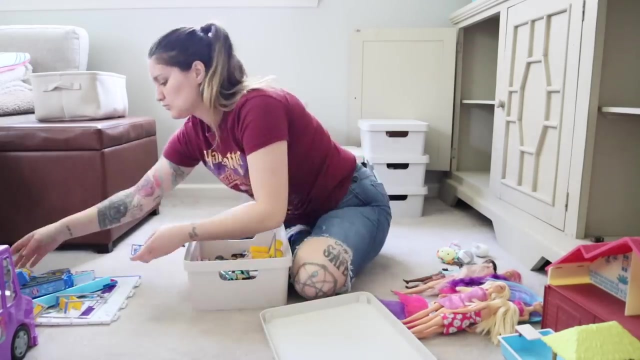 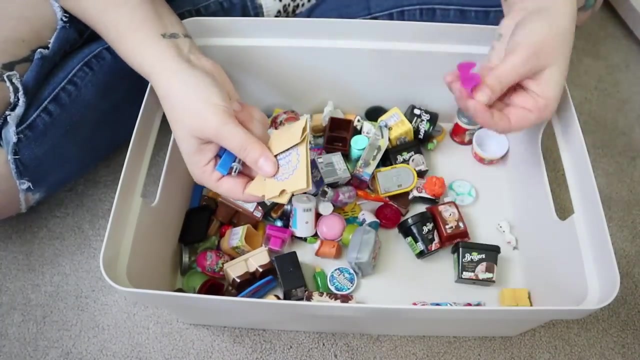 I do. they choose those more often, but once I do that, we'll start going through the rest and we'll try to even this out. so there's more in the declutter pile than the keep pile. you sorting through all of these teeny tiny toys is so tedious and mind-numbing and is probably the 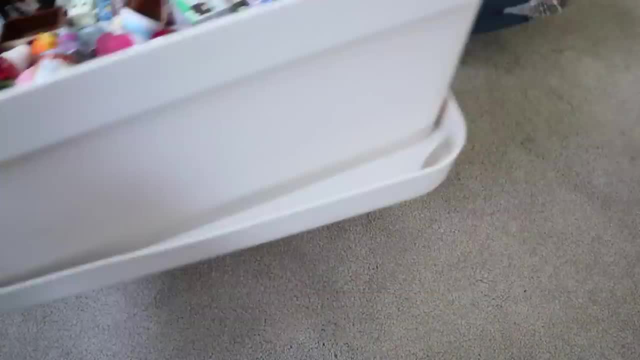 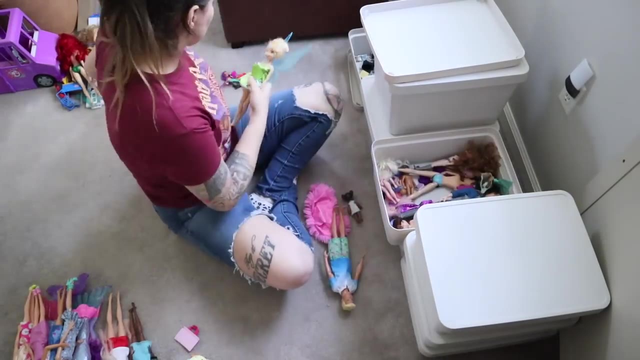 number one reason why I put off decluttering these spaces for so long. it just becomes so fatiguing for me and I feel like if there's anything that I want to do, I'm going to have to time during this entire process that I feel like I could just get up and walk away from it. It would 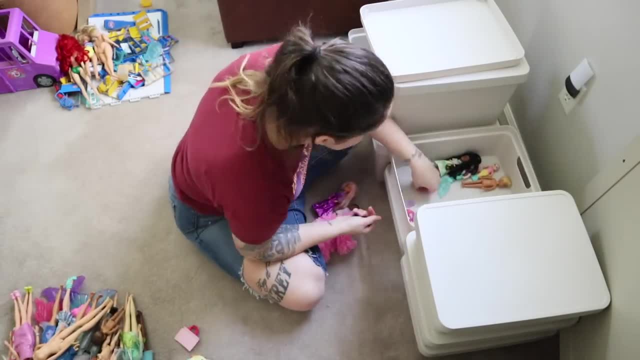 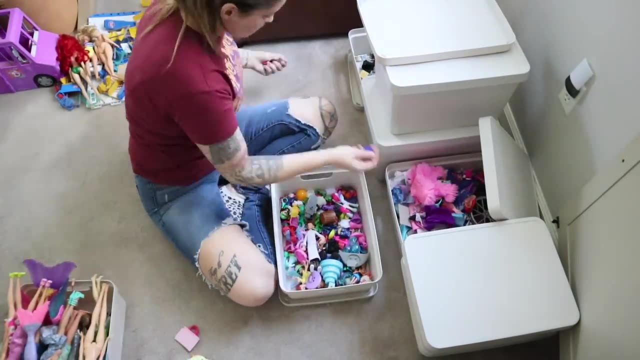 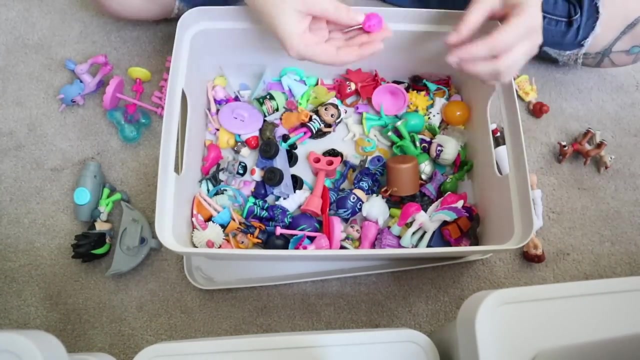 be when I'm going through all of these bins of super tiny toys. So what I've started doing is, before I go into a big declutter or a project like this, I kind of come up with a game plan where I think of a minimum of five things that I know for sure that I want to declutter from that. 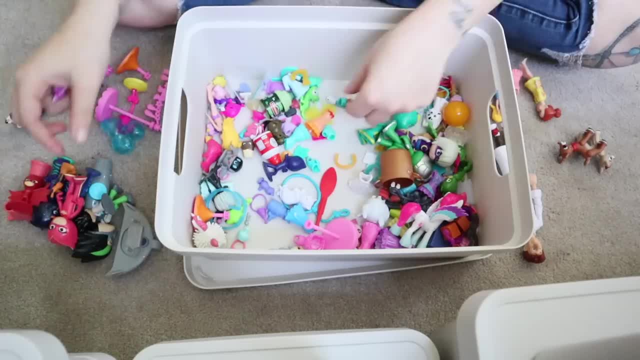 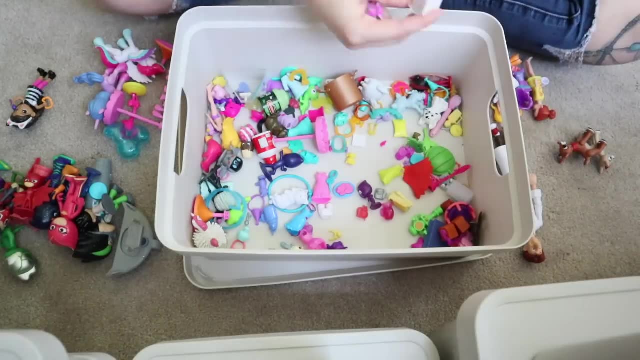 space and declutter from our home, And so then, when I'm going through all these tiny little bins, it feels like I have an intention or a purpose behind it. I'm looking for something specific, and it makes this sorting more manageable and just easier to get through, because I know that. 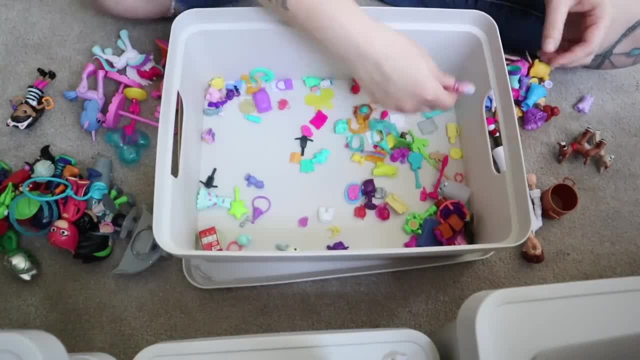 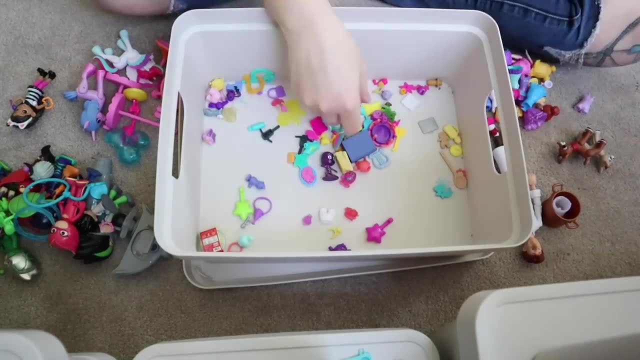 there is intent there and there is a purpose, and I've got a goal in mind, And so then I push myself to get through it so that I can achieve that goal or exceed it and keep making progress. So I just wanted to share with you guys a little bit about what I'm doing. So I'm going to go ahead and 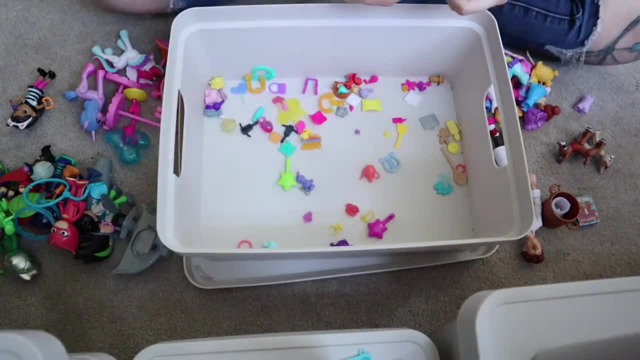 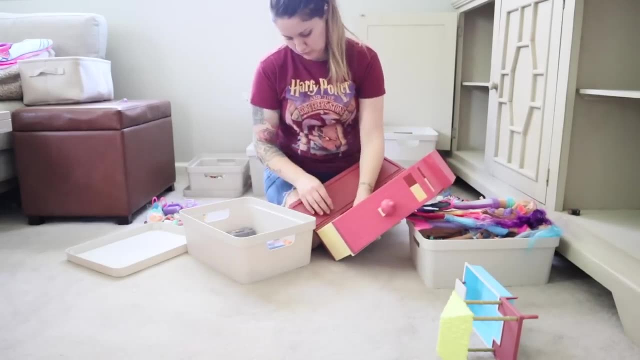 and I'm going to go ahead and show you guys a little bit about what I'm doing. So I'm going to go to share that in case any of you struggle with those little tiny tasks that kind of catch you up and cause you to completely avoid doing something like this or move it from your to-do list day to 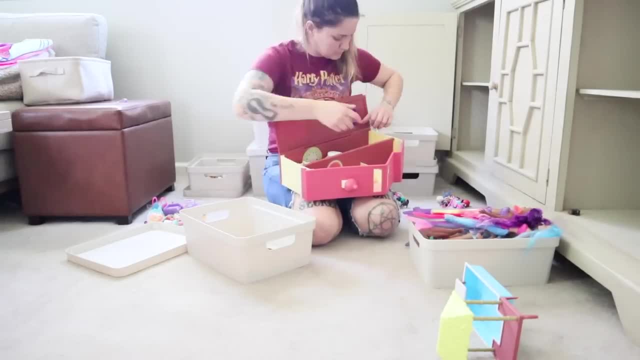 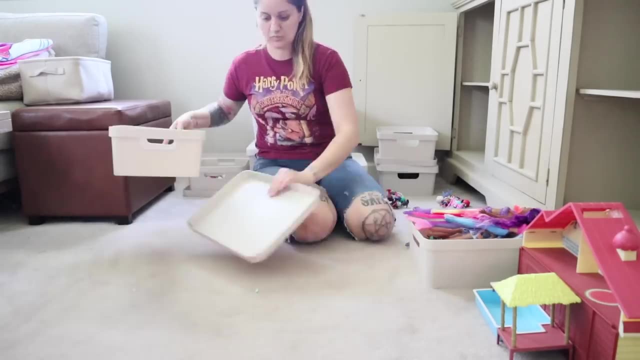 day but not actually get it done. If you struggle with that, like I do, hopefully that tip helps you. You'll have to let me know if you can come up with a game plan- at least five things in mind that you know you want to declutter, and if it pushes you through and helps to motivate you to get through. 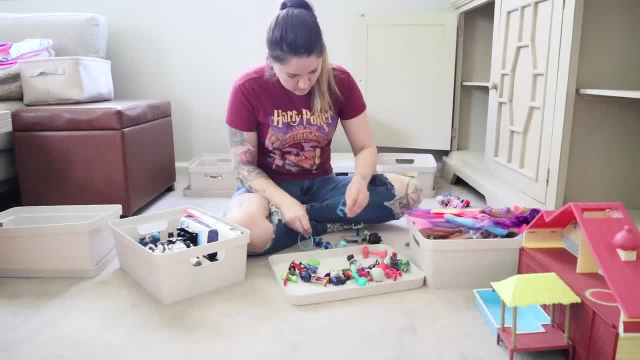 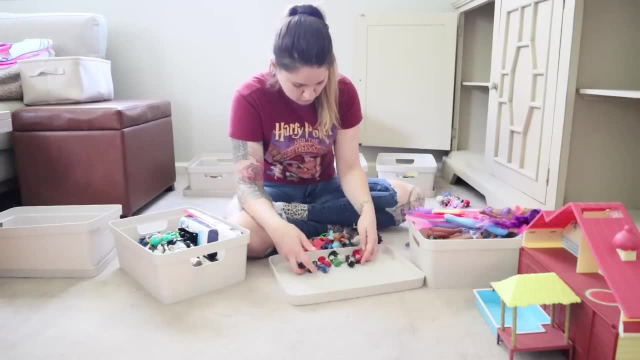 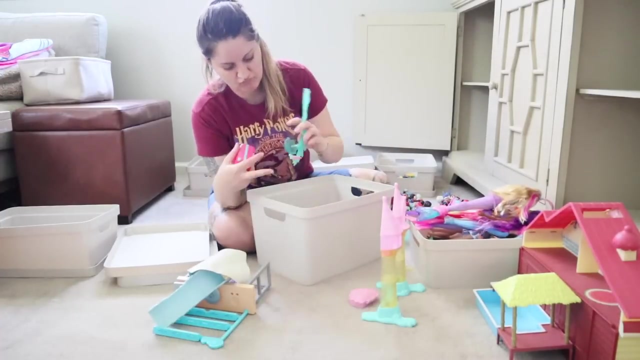 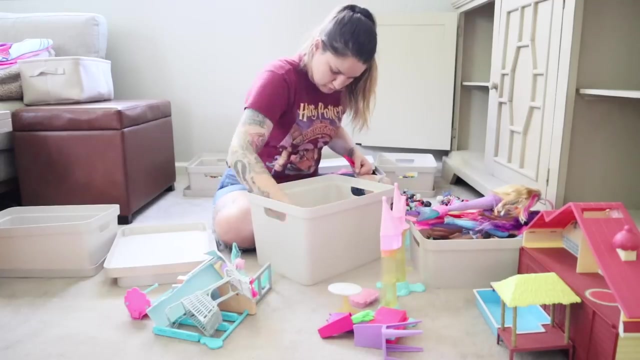 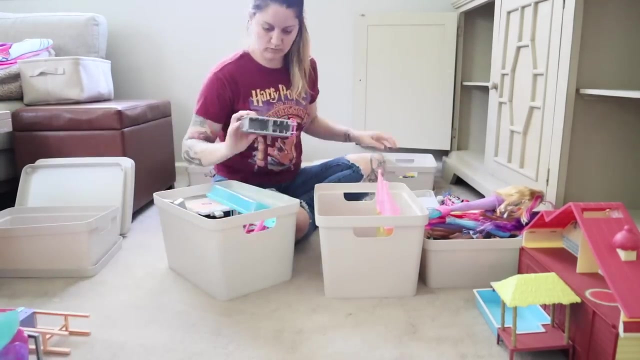 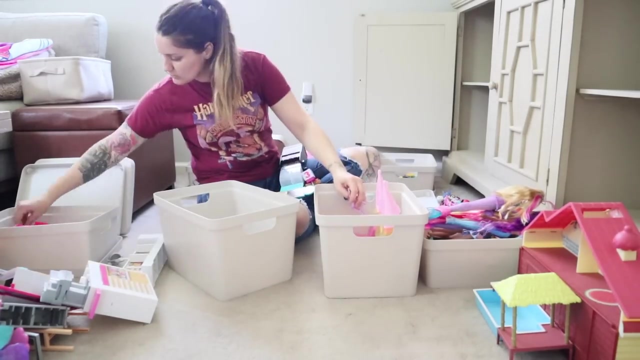 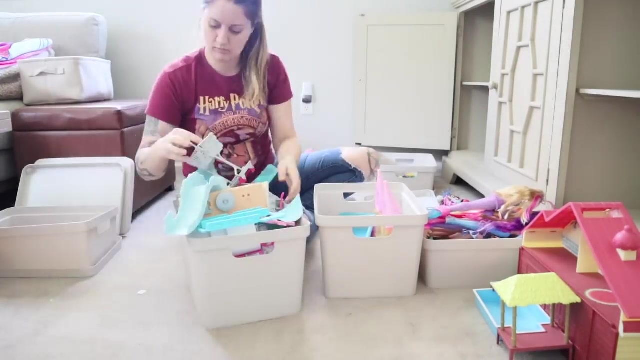 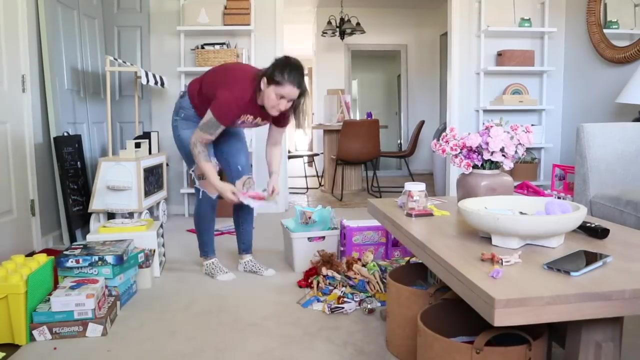 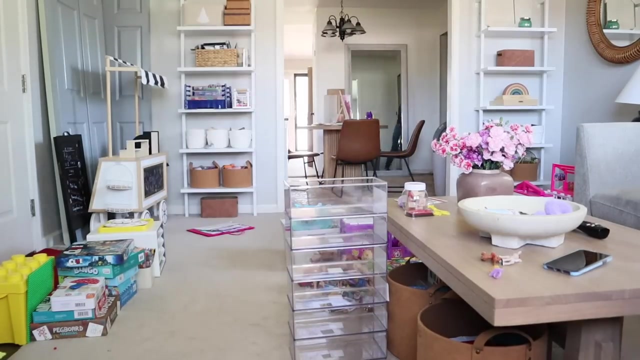 the rest of that task. So I'm going to go ahead and show you guys a little bit about what I'm doing. So I'm going to go ahead and I'm going to go ahead and show you guys a little bit about what I'm doing. So I'm going to go ahead and 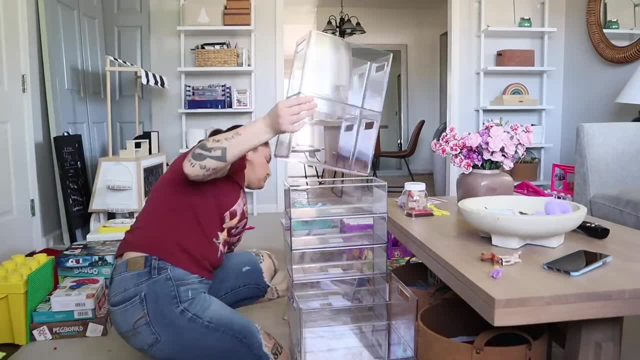 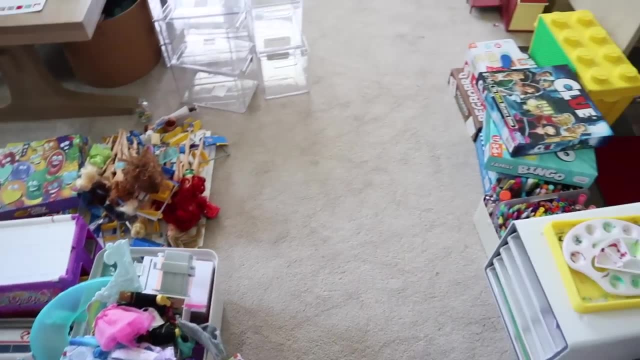 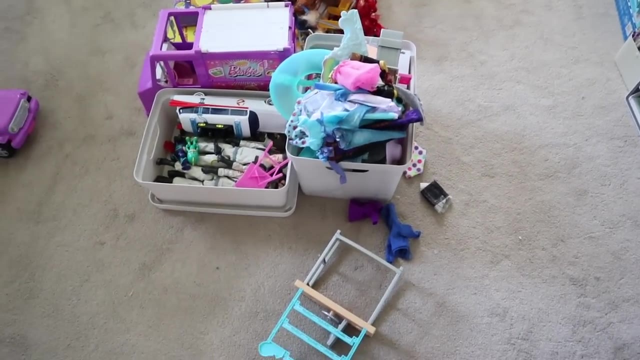 Okay, this is looking a lot better. It's definitely not like even with what we're keeping- Here are the things that we're keeping- but it's looking so much better. It's a really good start, because I still have some other areas to go through, but I've just got some Barbie, like clothes and accessories. 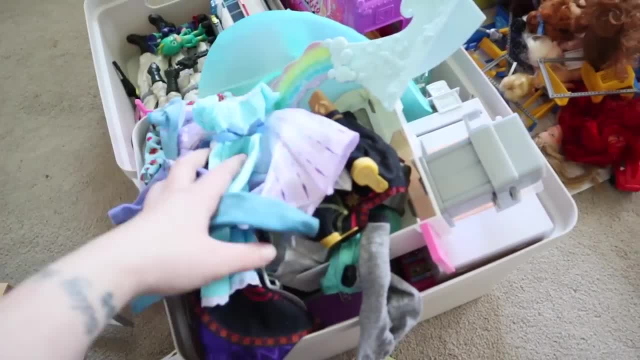 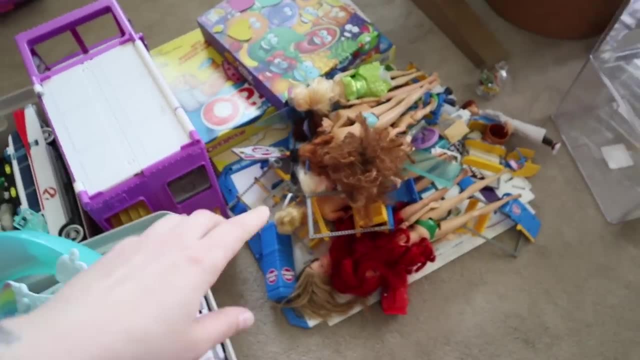 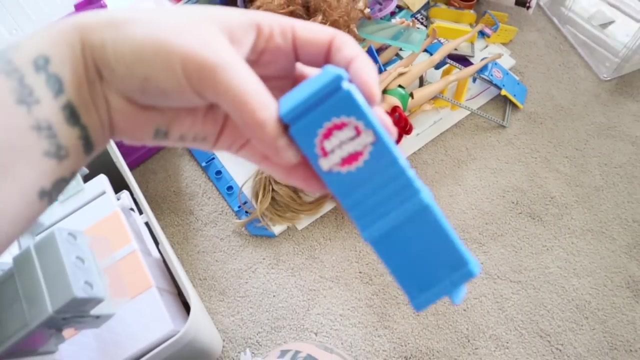 here larger toy play sets that I never see the girls play with. So we're going to declutter those. some other toys, the Barbie food truck, those games we already talked about, And then these are just some Barbies that we're going to be decluttering. And then underneath is this like little brands or 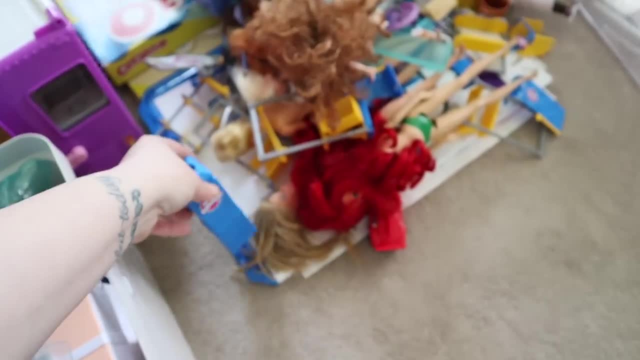 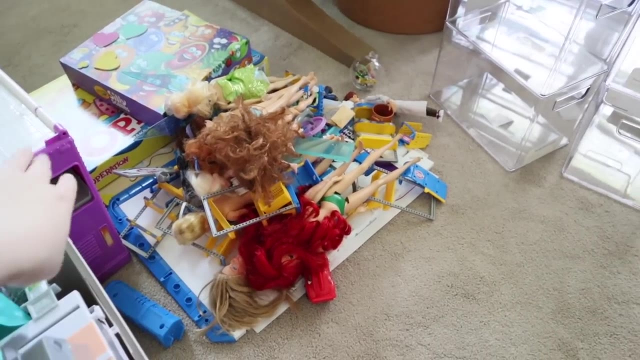 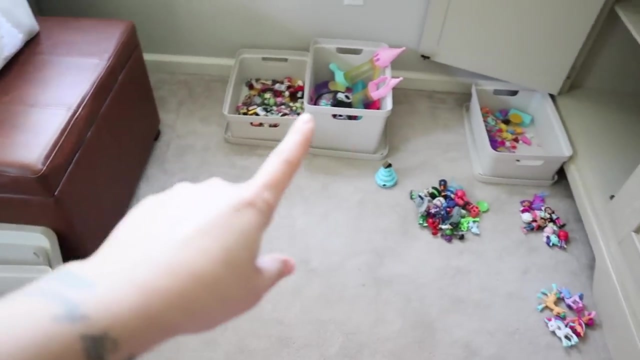 mini brands- I think it's called grocery store- that they set up once and it was a lot of work. So then they never set it up again. So it's fine, We're just going to go ahead and move on, declutter it, And then these are everything that we're keeping. One reason why this organization. 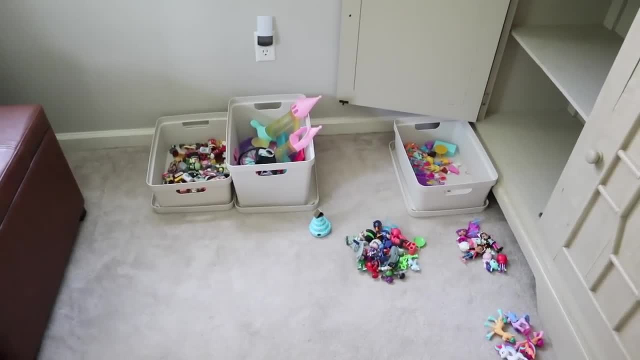 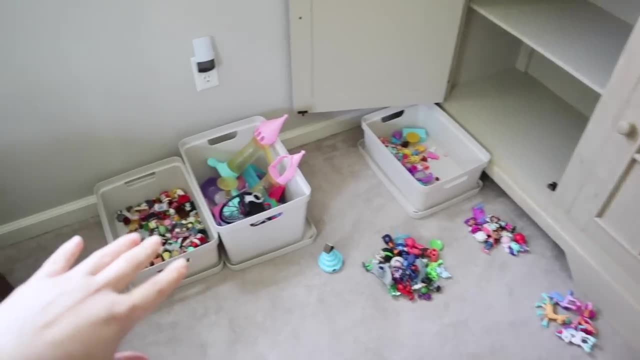 failed. I love the bins and I am going to keep them, probably for a toy rotation system. But one reason they failed is you couldn't see into them. So the girls like never wanted to pull them out, because they'd have to pull out everything to find what they were looking for. 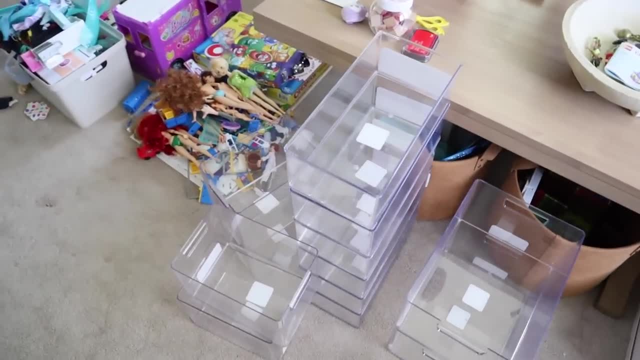 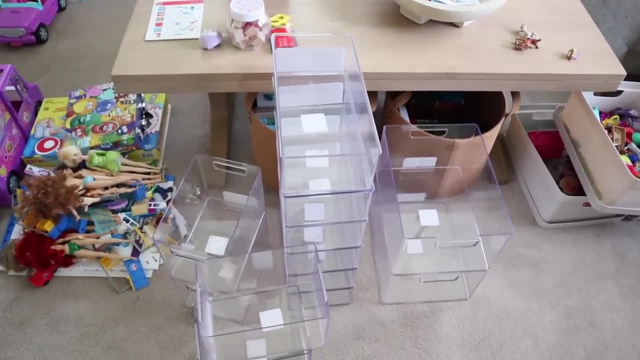 I got some acrylic bins from Target. These are all so affordable. I'll link them down in the description box. If you're looking for some acrylic bins for toy organization or any organization. they have such a variety of sizes So I'm going to go ahead and get them And then I'm going to go ahead and 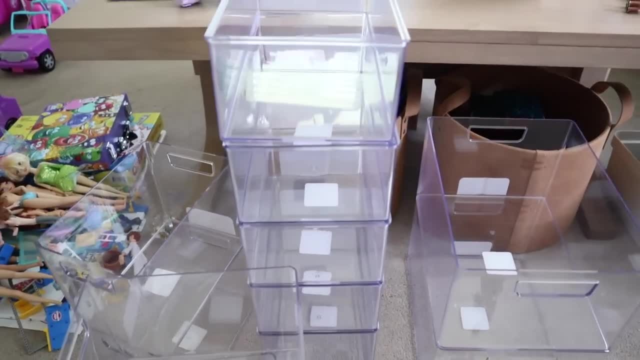 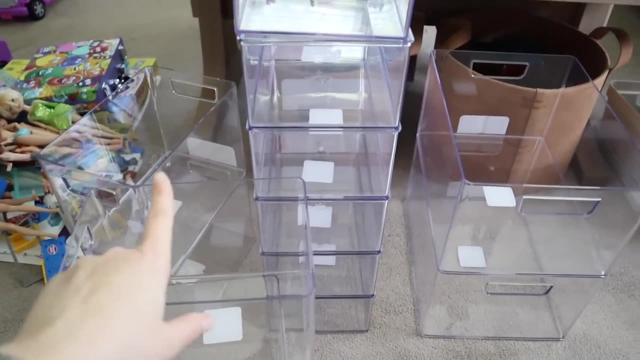 get the boxes here which I got like three sizes and they all stack, which I really like. But anyway, I picked these up from Target. We're going to see if these work out better and if they can be like micro organized kind of. So I got some of these. they al stack And I thought they'd be. 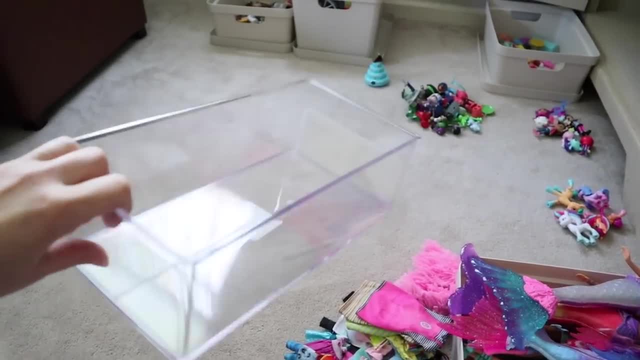 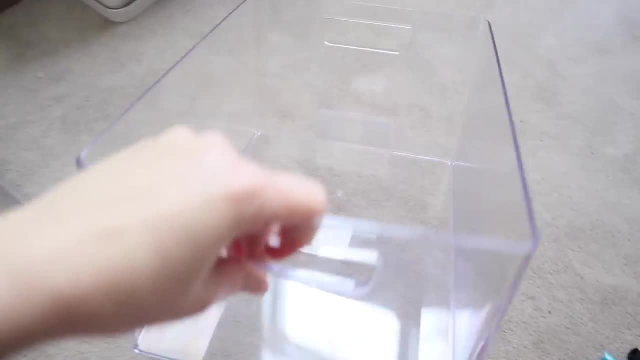 great for like these little sets of toys to put in here And then they can stack on top of each other. The girls will be able to see which set is in which bin. And then I got these thinking the Barbies could fit in there. And these are just like the mini. like the mini, you know, the ones that are a lot more. 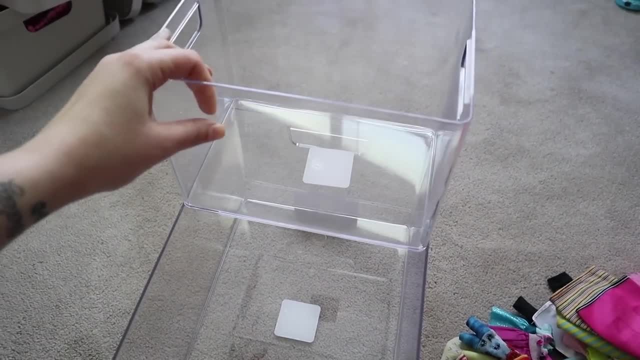 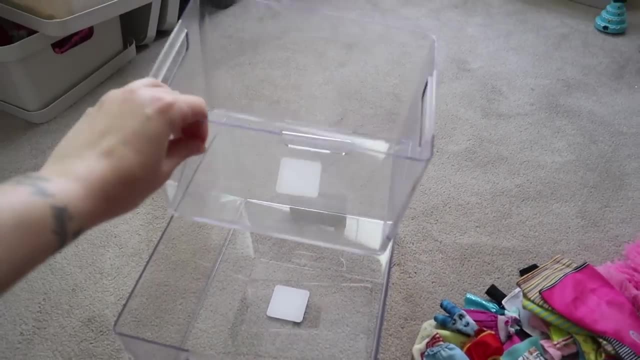 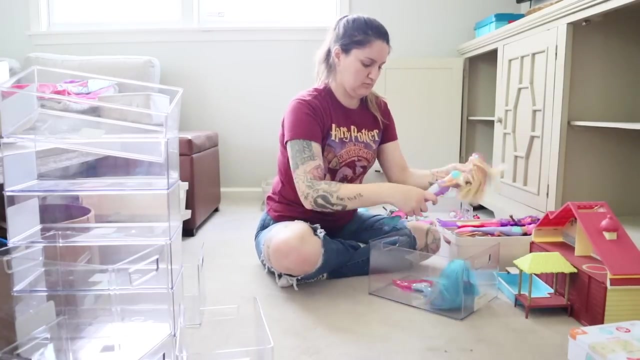 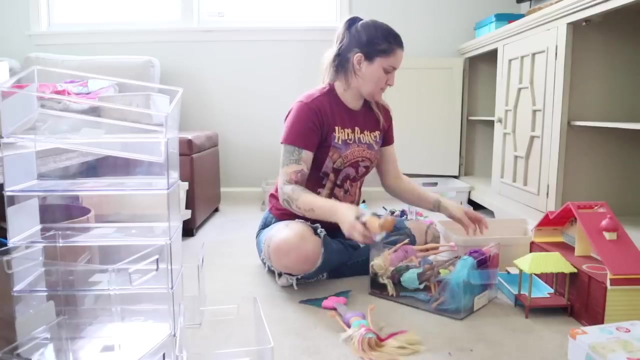 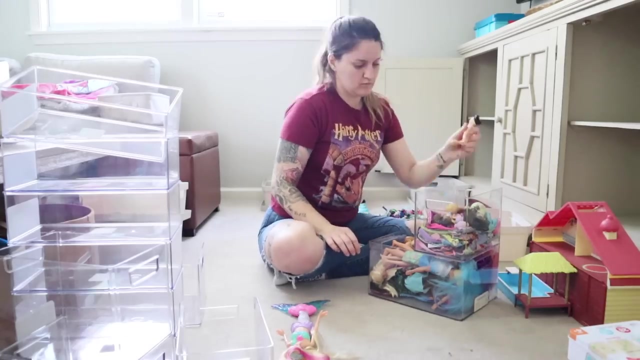 these that stack on top. I could fit like two on top of it, but one for like clothes and accessories and then Barbie's in the bottom. we'll see how it figured. how I figure it out, I am fine by myself, cause I won't be here alone. no. 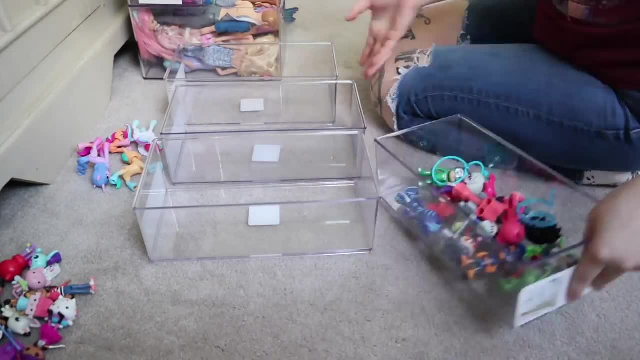 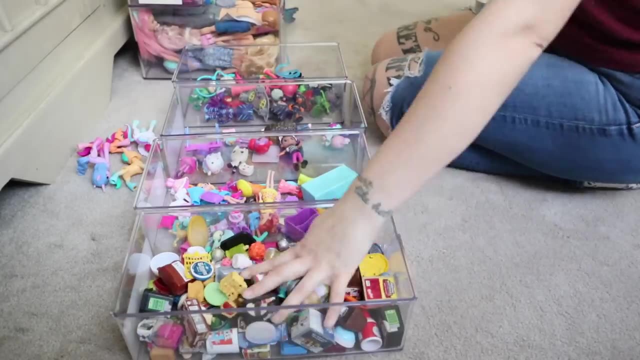 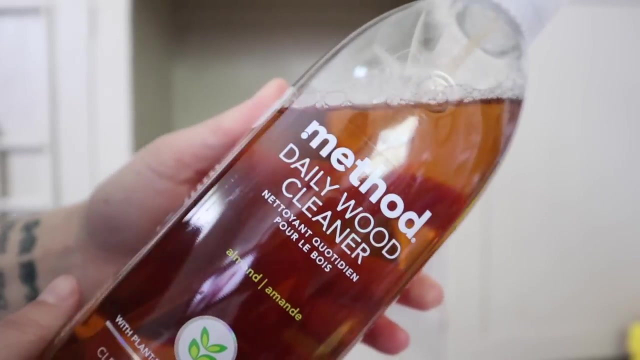 You don't know what you got. you don't know until it's gone. You don't know what I am worth. your words are like bullets now, Sometimes they hurt. I stay high when bullets fly. I am fine by myself, cause I figured how I figured it out. 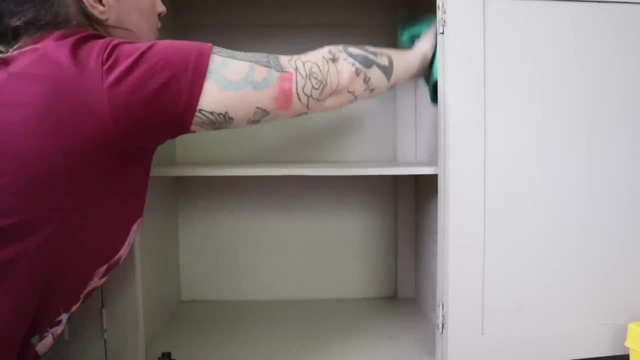 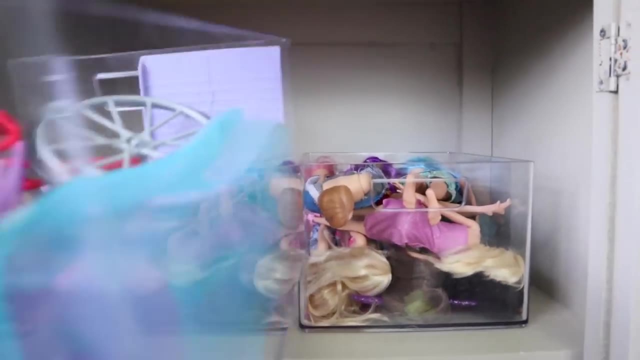 I am fine by myself, cause I won't be here alone. no, Out of reach won't be coming down. I can't wait till it's over. I can't wait till it's end. You got a pin on your shoulder and I don't need to pretend. 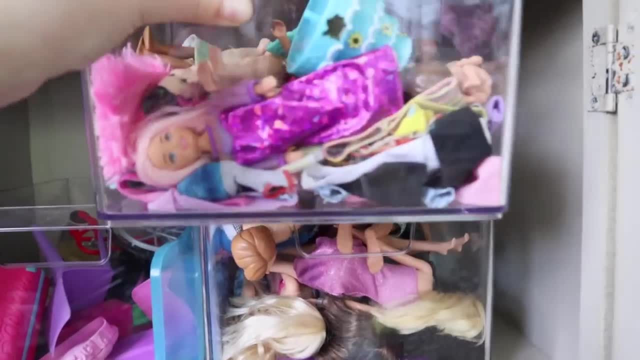 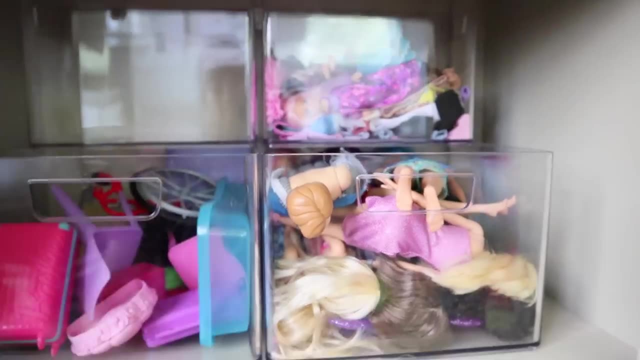 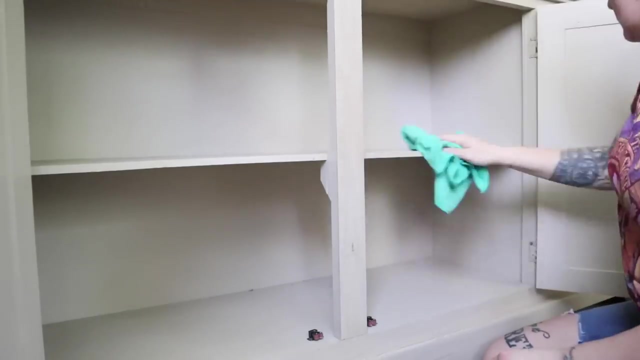 Yeah, we are alright, alright, We'll spend another night another night. I can't wait till it's over. I can't wait till it's end. You got a pin on your shoulder and I don't need to pretend. Yeah, we are alright, alright. 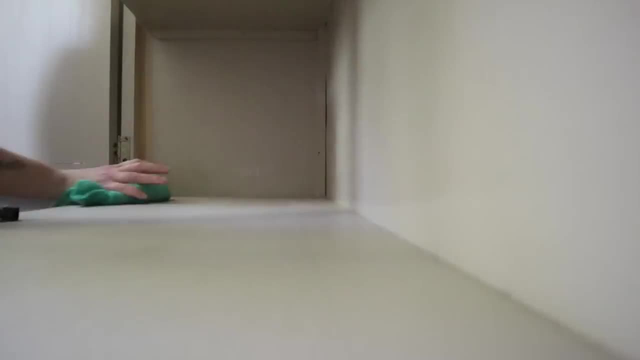 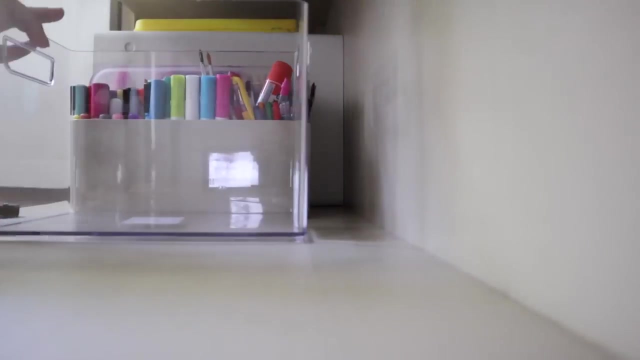 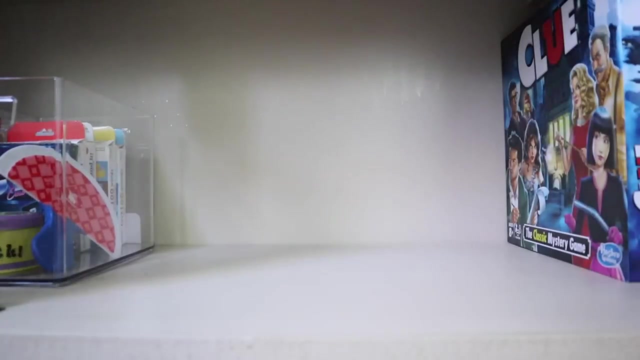 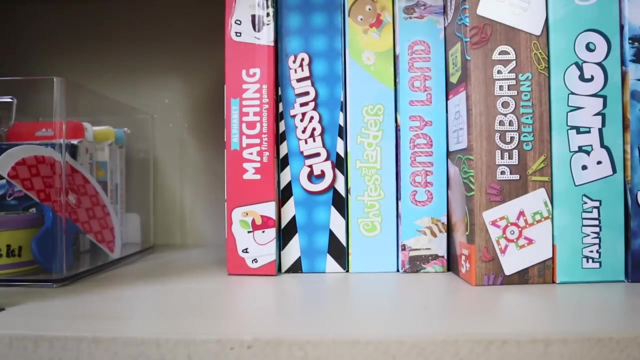 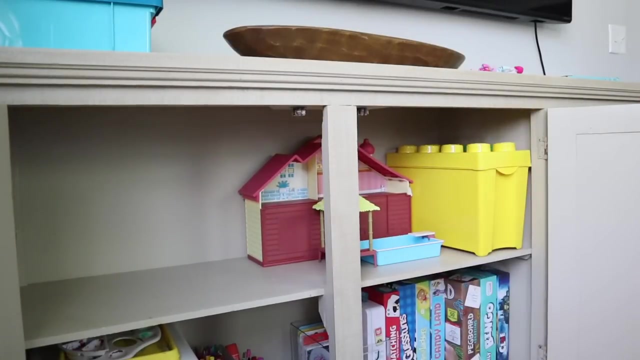 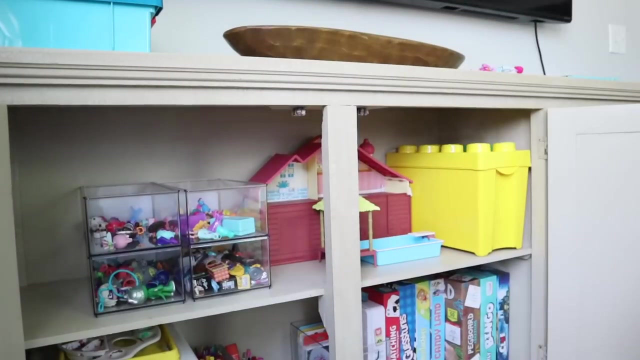 We'll spend another night, another night. I just wanna get lost. It's the only thing I wanna do. I wanna forget where I belong, I came from, where there's no getting over you. I am fine by myself, cause I won't be here alone. no, no. 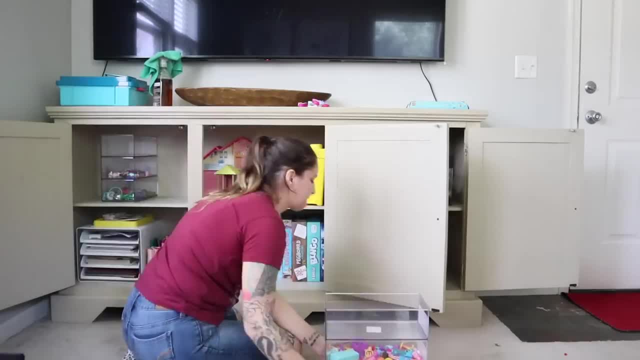 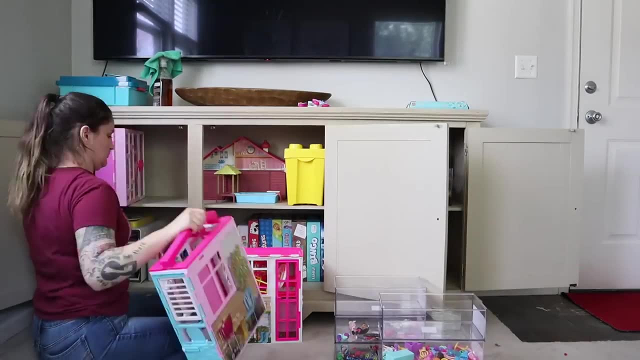 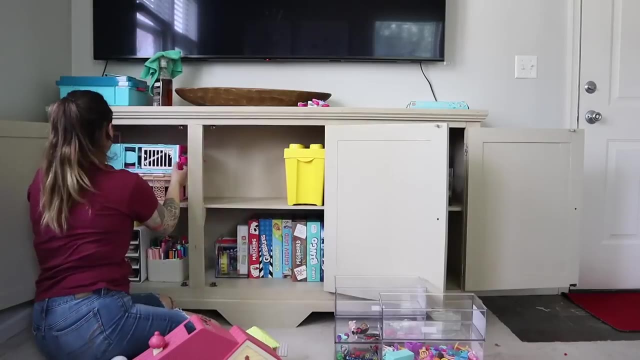 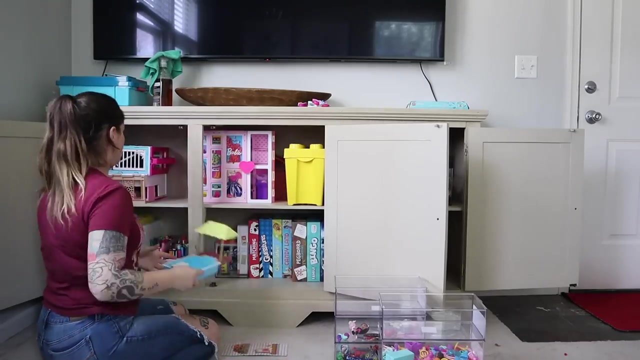 You don't know what you got. you don't know until it's gone. You don't know what I am worth. your words are like bullets now. Sometimes they hurt, sometimes they hurt. I stay high when bullets fly Out of reach won't be coming down. 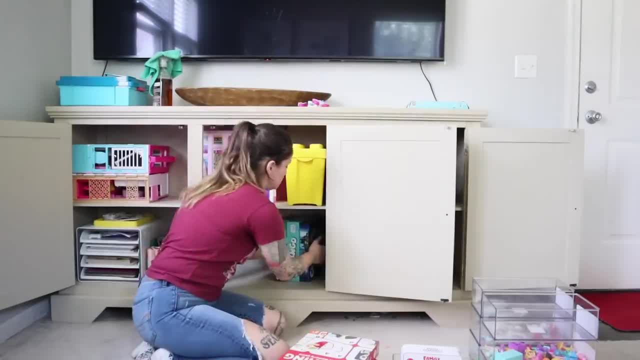 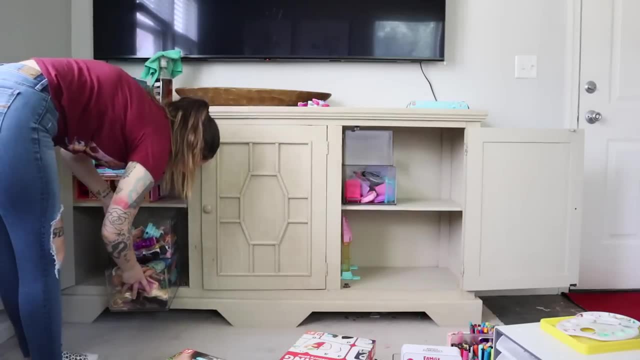 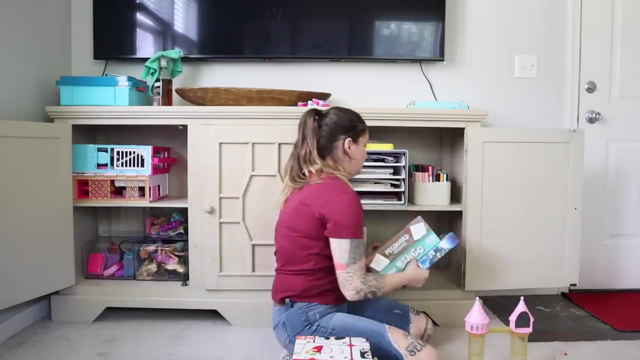 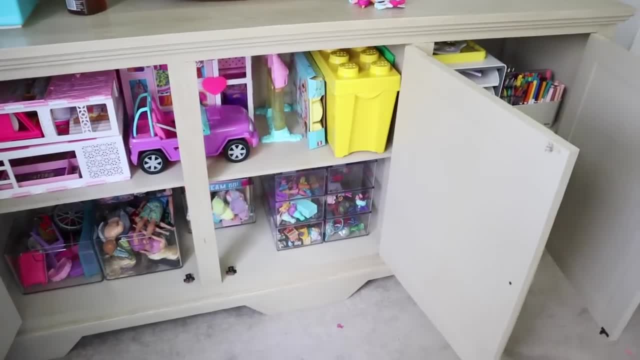 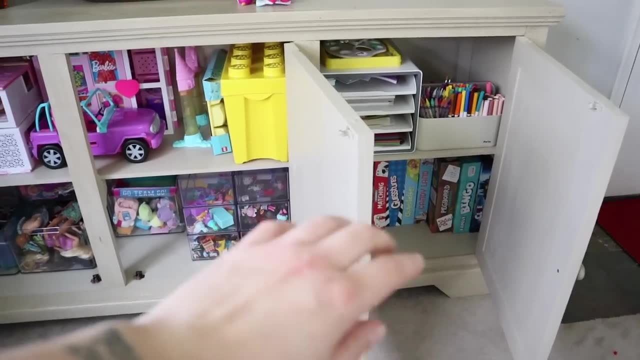 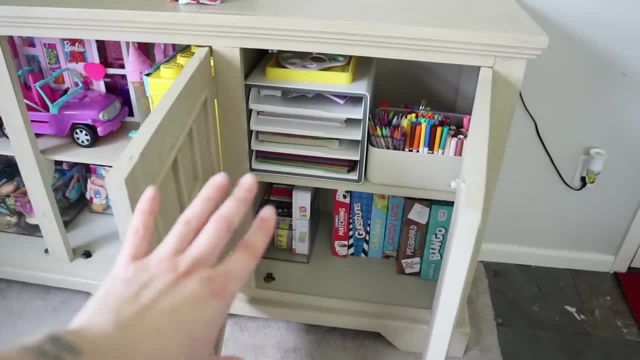 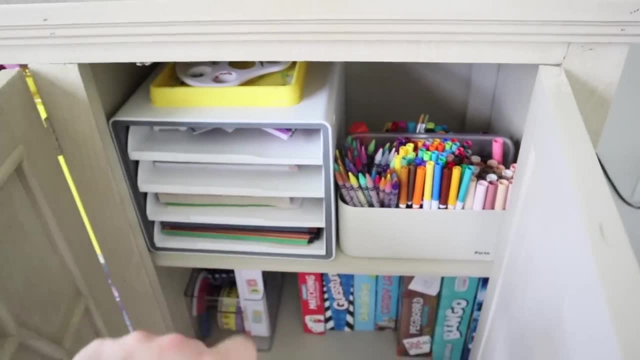 going to make this a Barbie cabinet, but it makes sense to just keep these things. So we have craft supplies, their caddy. I have room for an acrylic bin back there, so I think I'm going to add that for all of their jewelry making crafts. And then down here we've got all of our favorite board. 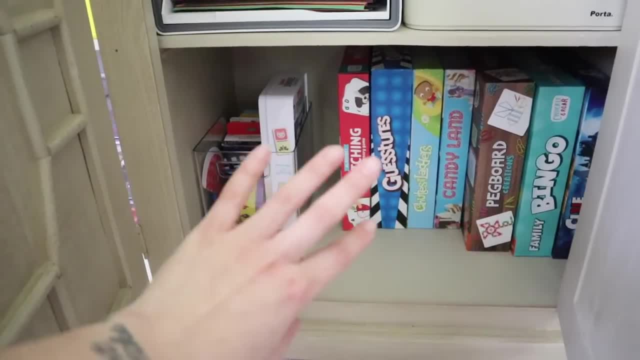 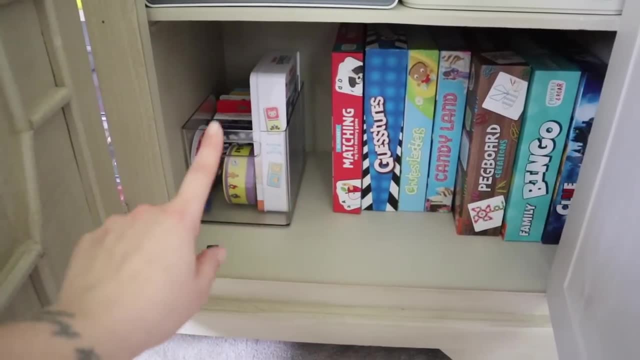 games and learning activities from Chuckle and Roar. That is like our most recent obsession. We love it. It's helped so much with Sawyer's kindergarten readiness, But anyway, there's room to grow. And then I have this with all of our card games and I think I might swap it out. 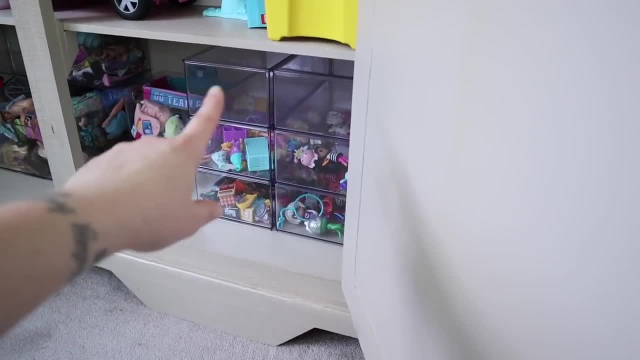 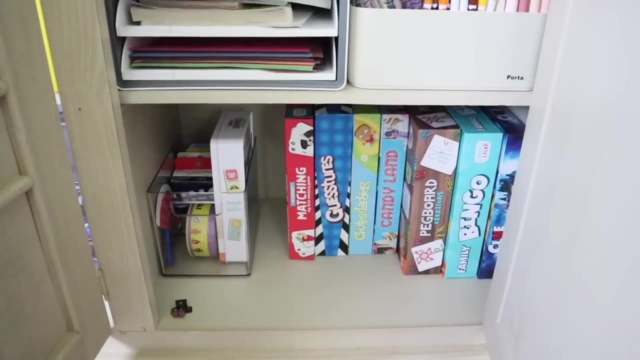 for a three stack of these. I feel like the card games would still fit in that top one, and then I'd also be able to add like kinetic sand and things like that, which we don't mind Sawyer having access to. So I think I'm going to do that. Derek's going to Target for me to like. 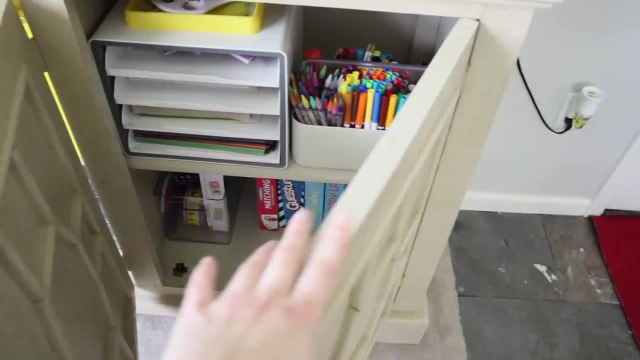 get some of that. So I'm going to do that. So I'm going to do that, So I'm going to do that. more acrylic bins, But anyway, there's all of our craft supplies: board games, and then over here. 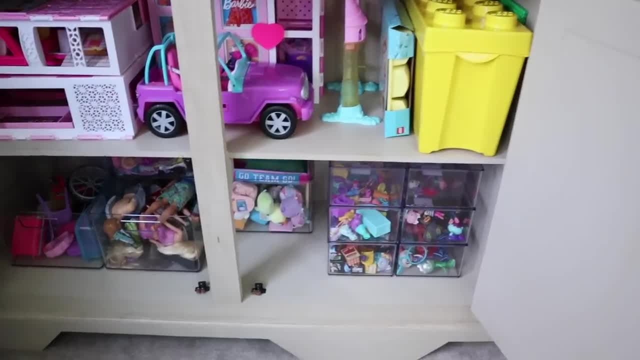 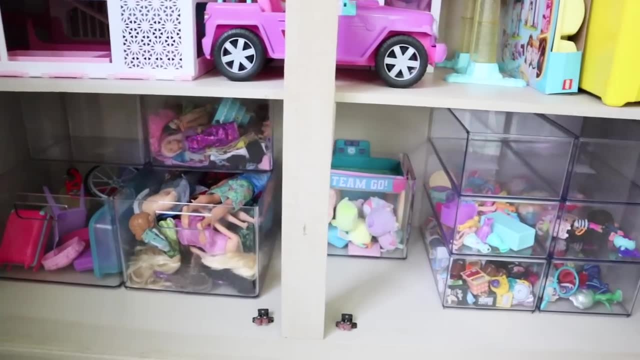 all of the larger Barbie toys and accessories, the Legos and then, down here, all of the acrylic organizers. This worked out really well. There's some empty ones and empty spaces, so there's room to grow as I go through the rest of the room, which we are about to do now. So 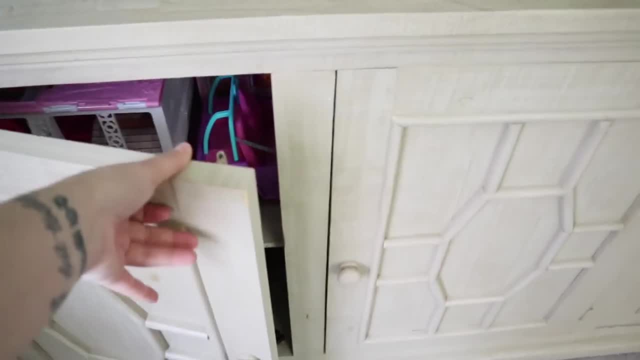 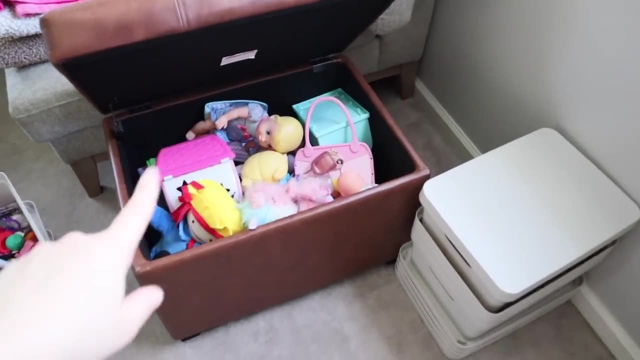 I'm going to shut this for a second, since I've got this under control for now And we're going to move on to some other areas. So my goal is to sort through this and completely empty it out for all of the girls, WWE wrestlers and wrestling ring, because that takes up a lot. 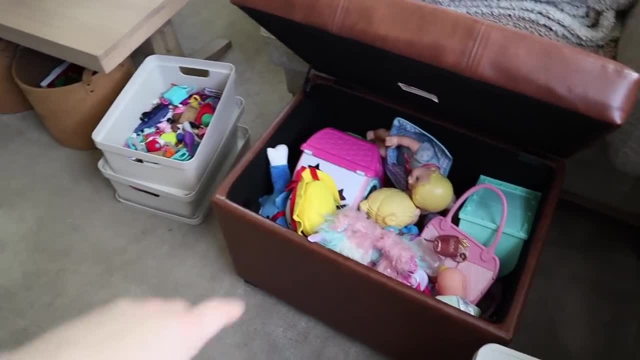 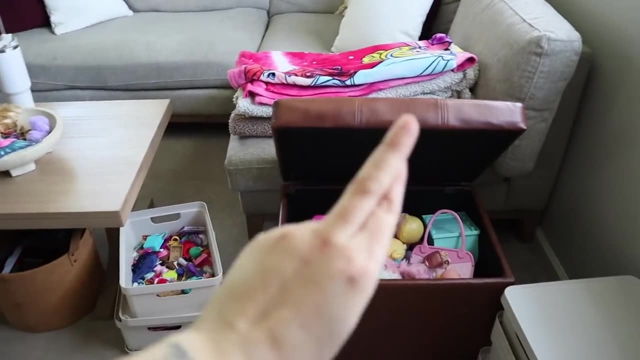 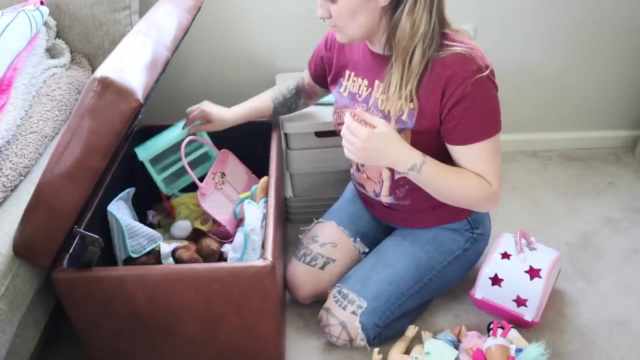 of space. Hopefully this is all just misplaced and can go to other rooms And then we'll move on to like the ladder shelves that are out of control and stuff. So wish me luck. Hopefully we can get this cleared up. Okay, so I can't lie. It has been so long since I have gone through. 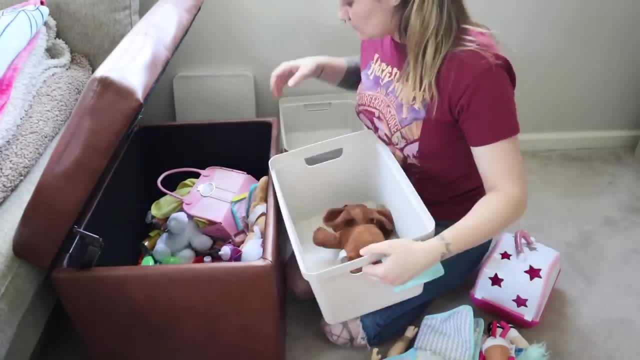 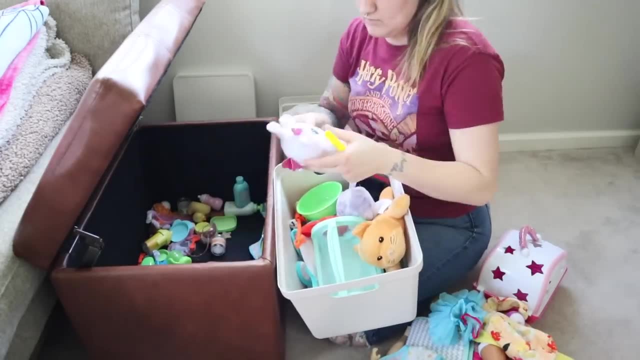 the storage ottoman. Initially, when I had set up this room, we used it to house this like Melissa and Doug brand animal vet rescue playset, and then a baby doll playset, And that's all that was supposed to go in there. But while I was sorting through it I realized that this had just 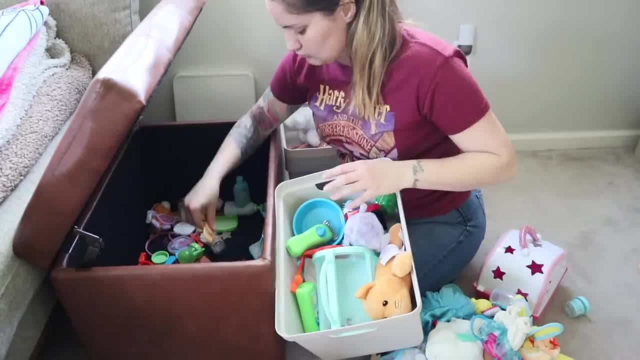 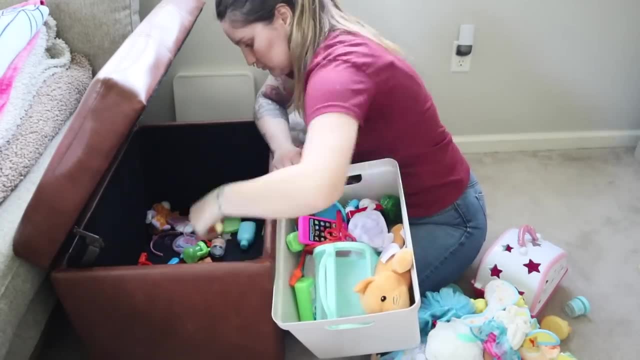 become the black hole of toys that didn't have a home. So it took me a little bit to sort through it all. I ended up having that one bin in my lap of donations and then everything else was just out of place and needed to be put back where it belonged, So I went ahead. 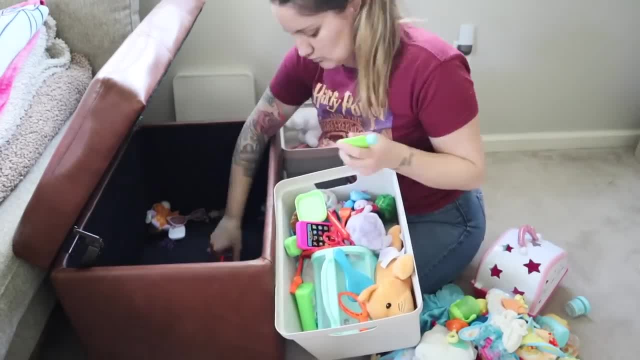 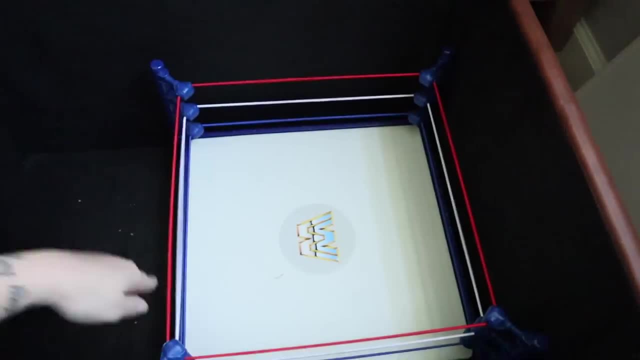 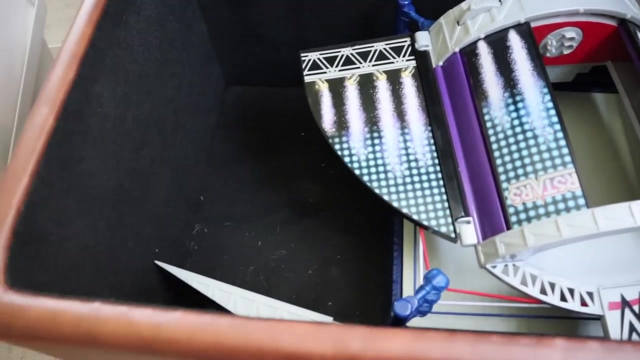 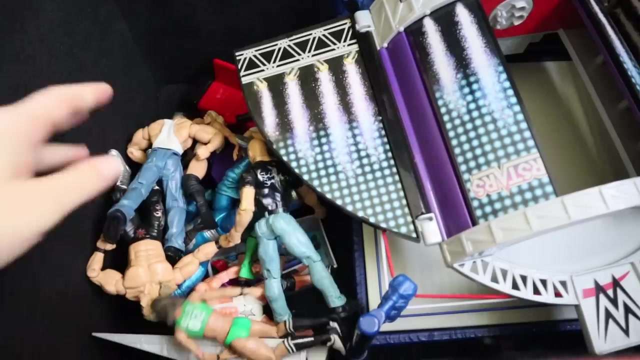 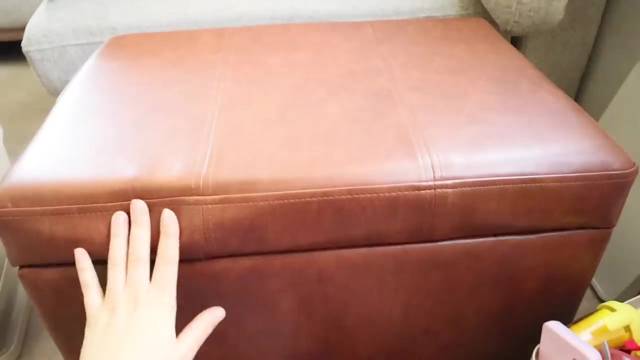 and did that. There was plenty of space to fit all of the girls, WWE figures and wrestling rings and all of their WWE toys, exactly as I had hoped for. Moving over to this market cart similar to the storage ottoman, I did not realize exactly. 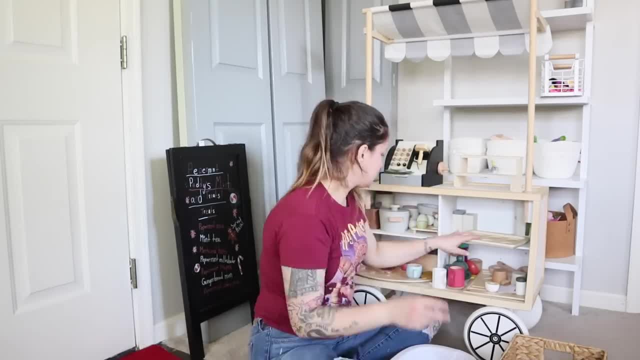 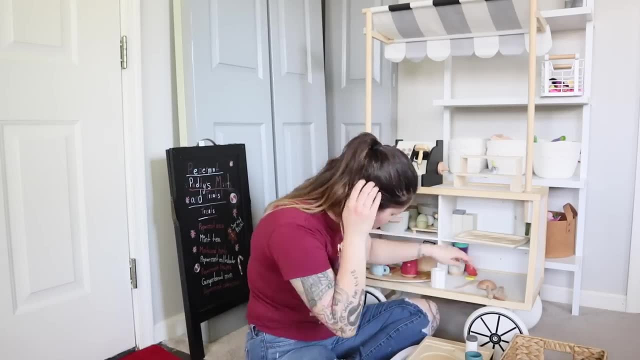 how much stuff had accumulated in this corner of the room And it was feeling overwhelming to me just trying to sort through everything, find all the pieces for each set and get it all set up. So I imagine it was feeling that overwhelming and stressful for my kids as 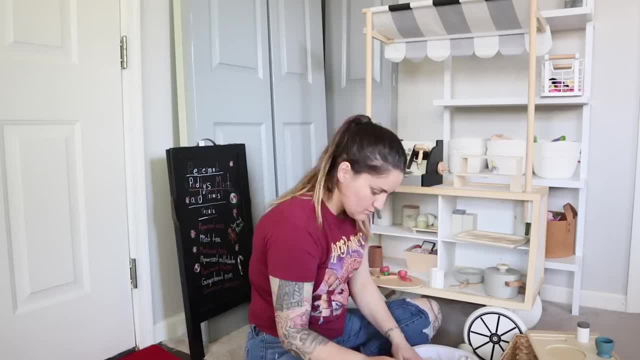 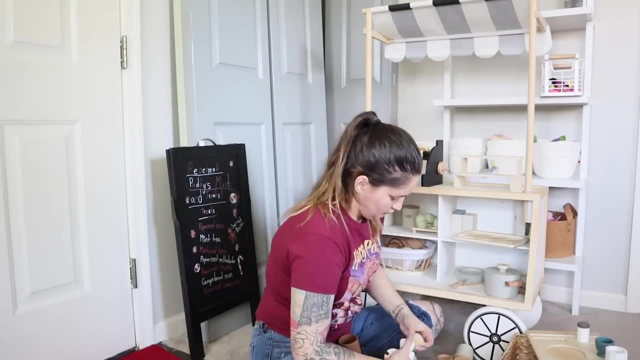 well, And I had seen them decrease the amount of time they were spending with this toy set in particular. So I made it a goal. I decluttered 50% of what was in here, simplified it a ton went with the less is more mentality. 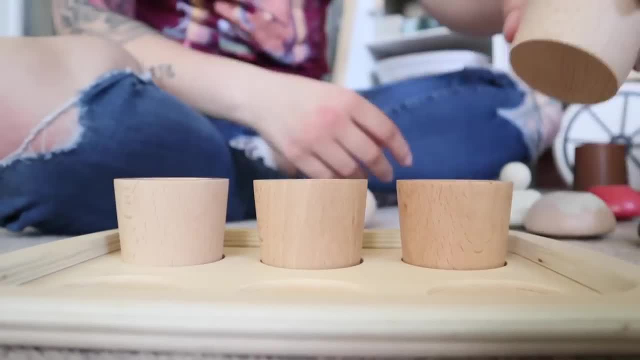 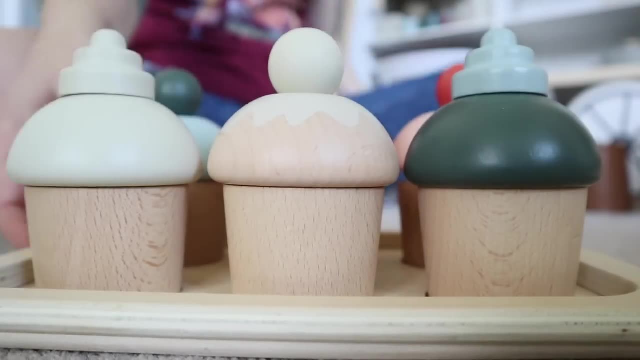 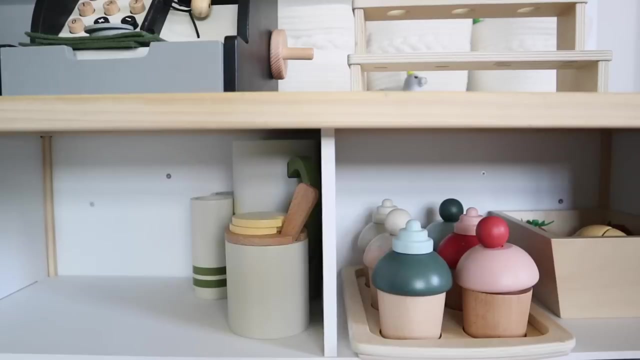 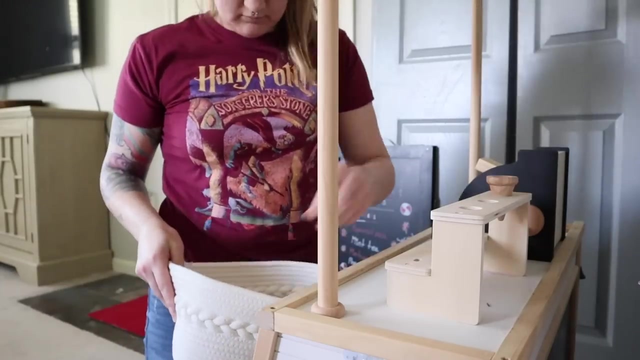 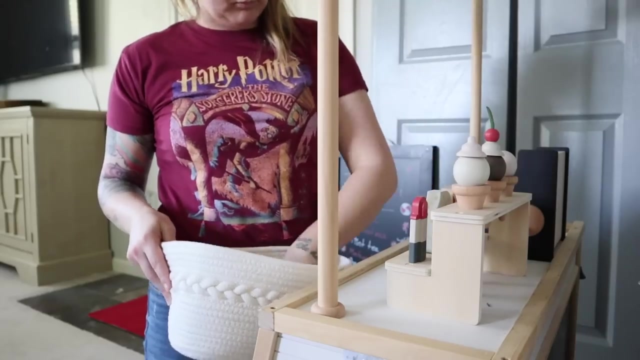 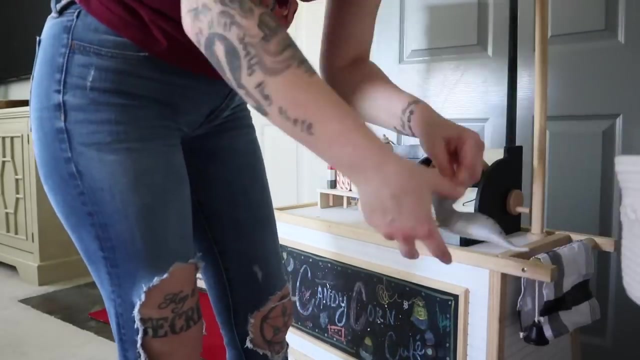 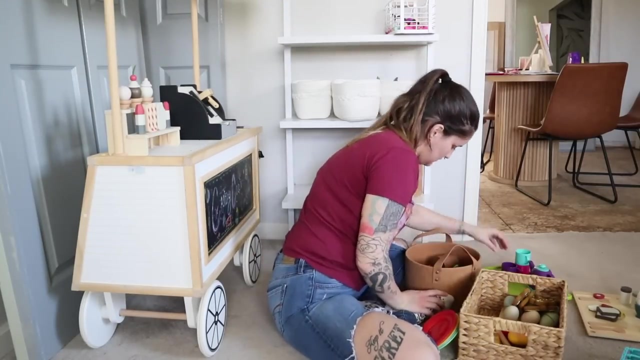 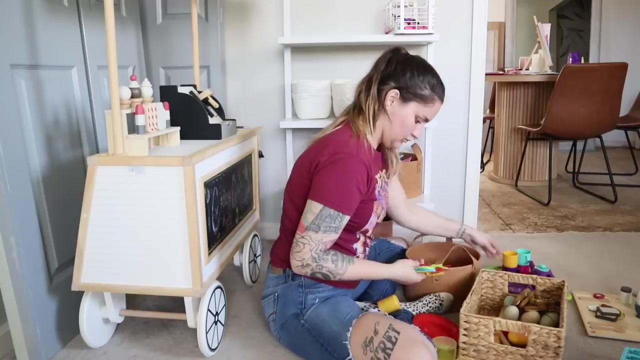 and that has been working out so much better for us. When I was initially working on trying to figure out this space and doing the countless makeovers that I've done in here- I swear I've changed my mind a million times, But that's just because I was never fully satisfied with what I was coming up with- the furniture- 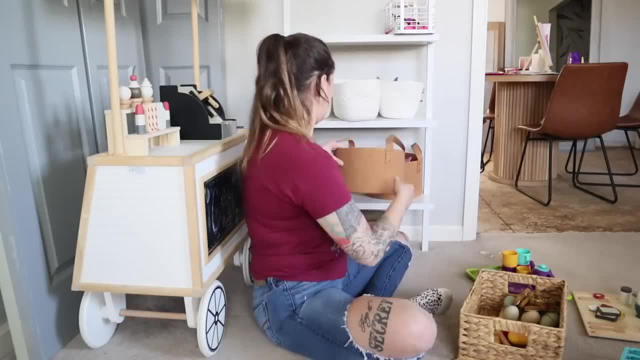 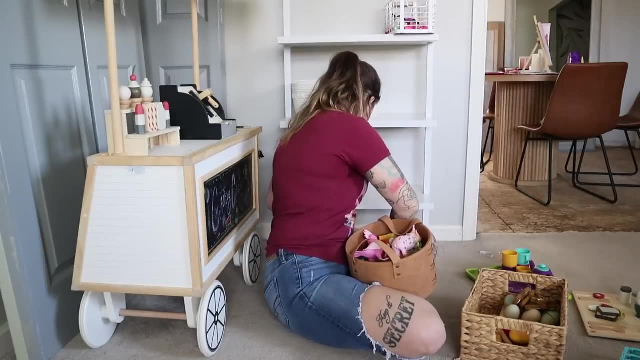 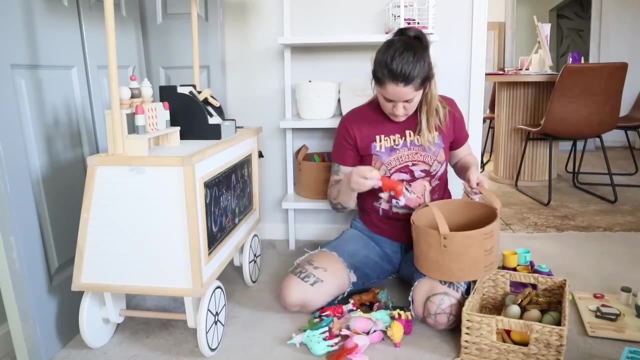 that I was bringing in here and trying to figure out the layout, But discovering these wall mounted ladder shelves changed the game for me. I love the way that they frame this doorway and they offer additional storage in these otherwise empty corners of the room, And then also on the upper shelves. I like to do more decorative items, So I feel like 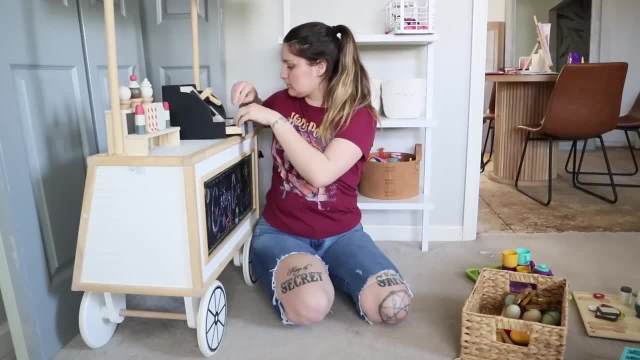 it's a really good in between and serves like an intention and a function in this space, And I just love them so much. So if you're thinking, Oh, I'm going to do these, I'll. If you're struggling with an area like that, consider these ladder shelves. 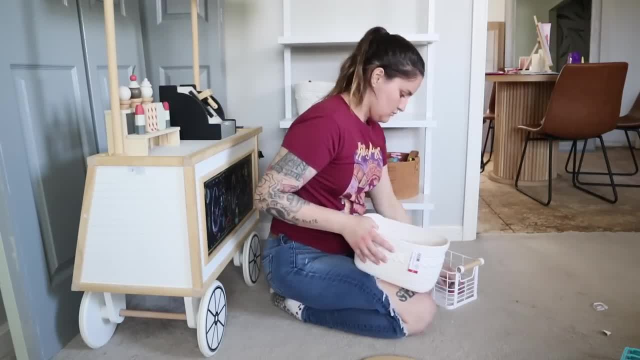 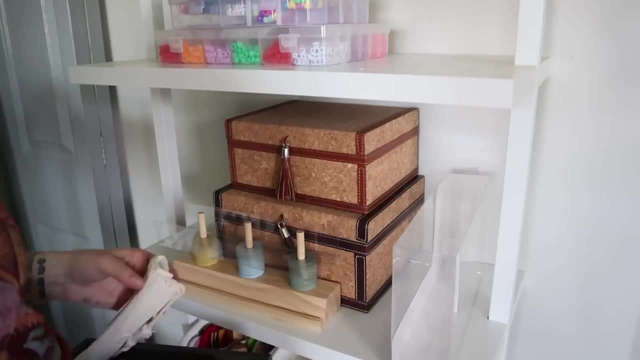 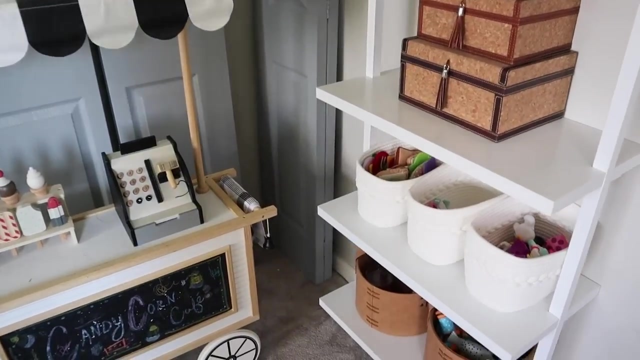 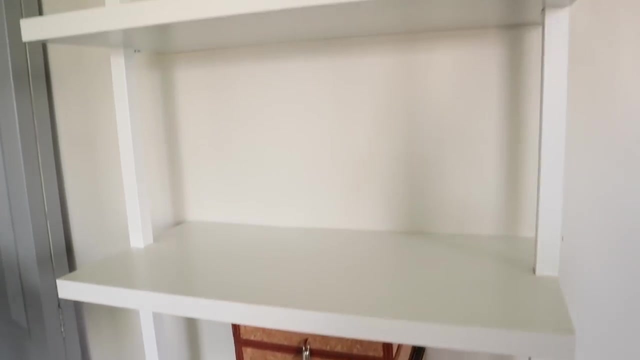 I'll leave them linked down in the description box in case you want to check them out. They are probably my favorite furniture purchase that I have ever made. Okay, this is looking so much better over here. I am very happy with this. I actually have some room to put out some like spring decor now. 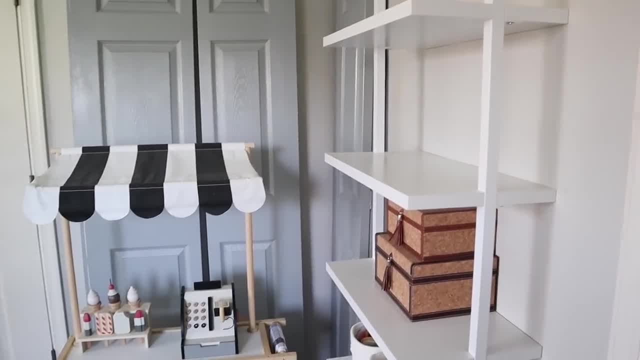 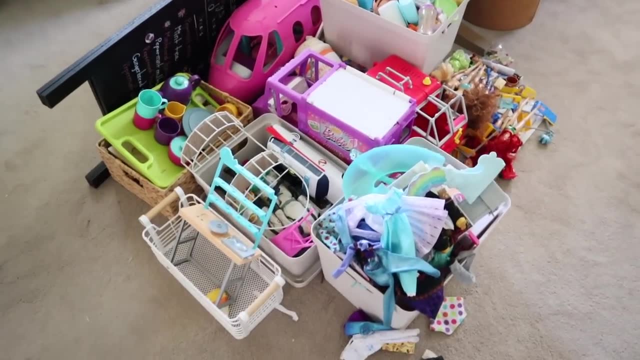 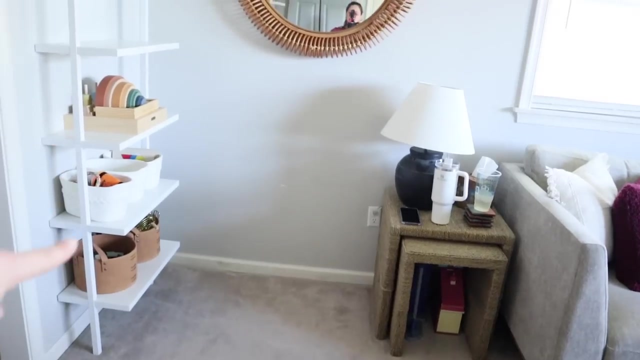 I haven't even like decorated for spring or Easter yet, because things have just been like piled everywhere, But now I can do that. Also, here is our massive pile of donations. I am happy with myself And, after having all of this organized over here, getting everything in there, organizing all of this, 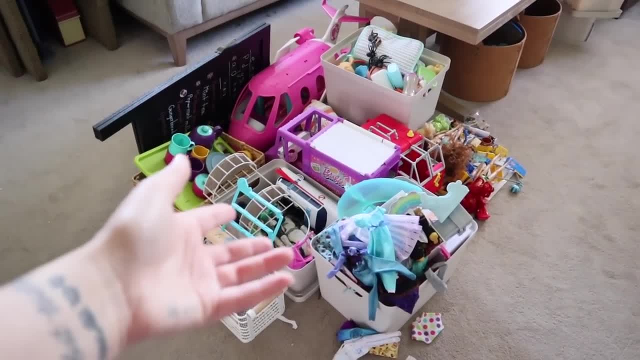 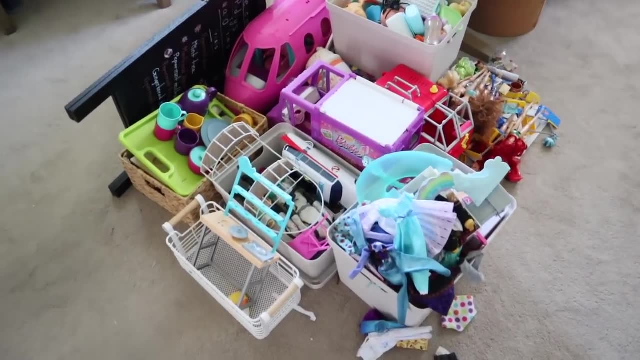 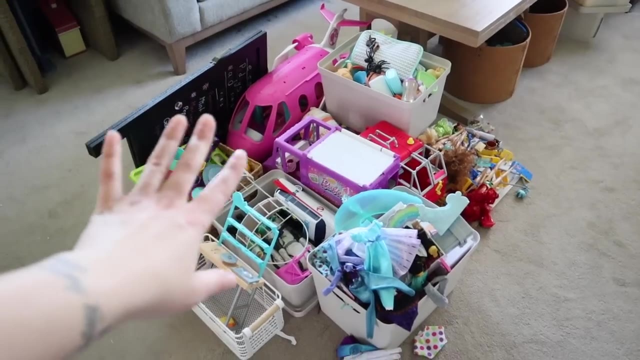 I don't know where this stuff was Before. probably it was the stuff spilling out everywhere and like not actually having a home, because I could not if I wanted to find a home for every single one of these items in this room. So it's got to go. 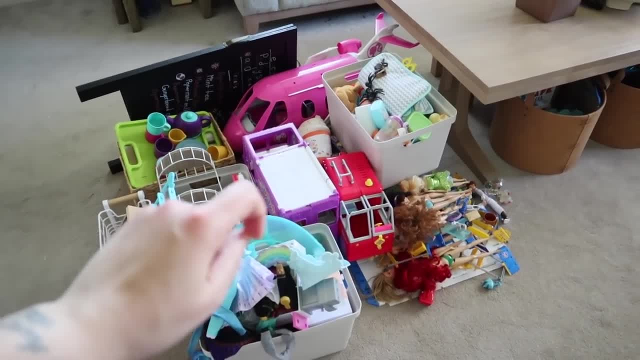 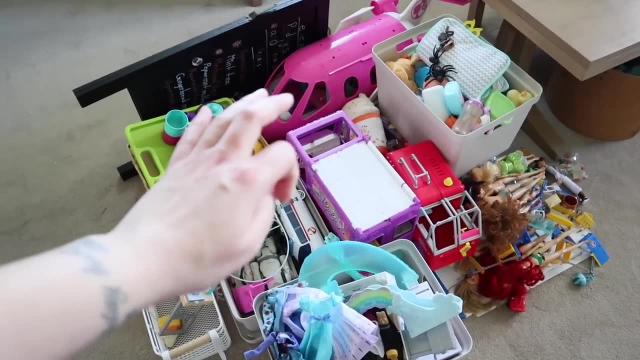 Just no hesitation. We're going to be taking this to Goodwill today. Well, actually we'll probably take it to the Women and Children's Shelter first, Anything that's in like really, really good condition If they've got like kids there currently. 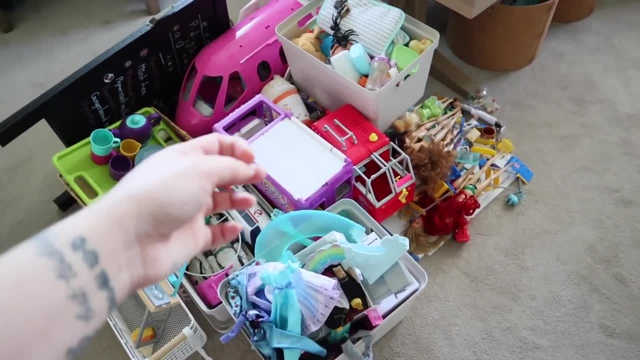 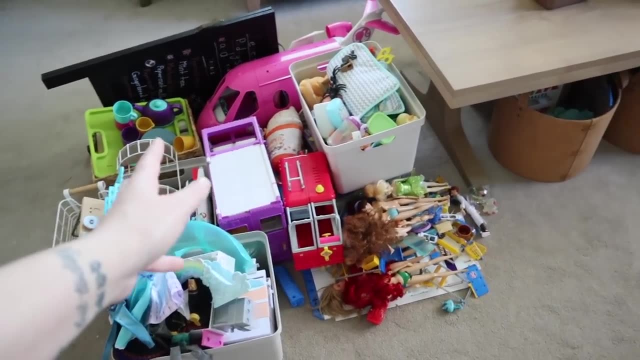 That could use this, because sometimes they do refuse donations depending on, like, the gender or how many children, the age, things like that. So we'll check with them first, Then we'll go to Goodwill if we can't take it to the Children's Shelter. 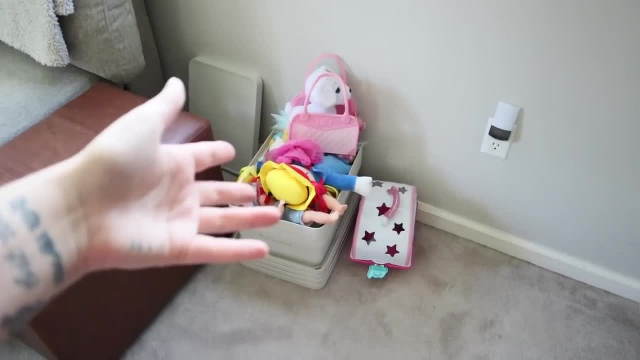 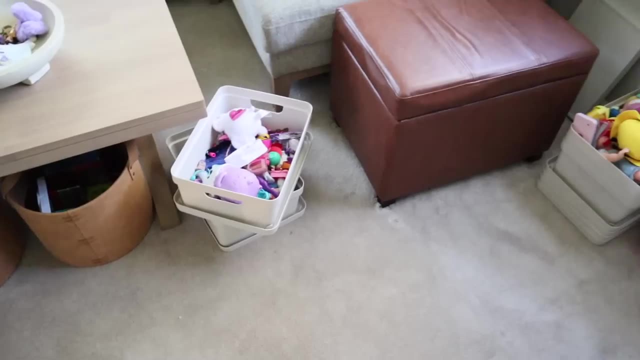 These things were just out of place. They need to go in Sawyer's room in her like stuffed animal bin And then these are the two bins that the girls need to go through when they get home from school. But other than that, everything is done. 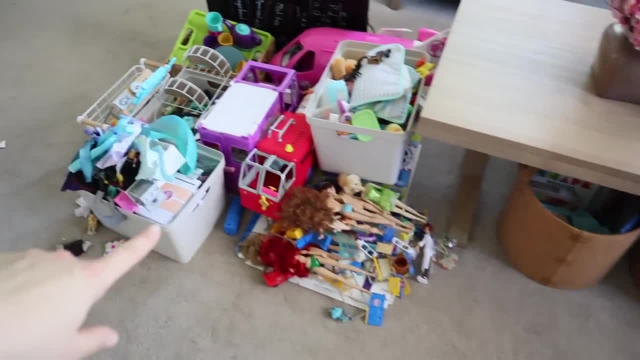 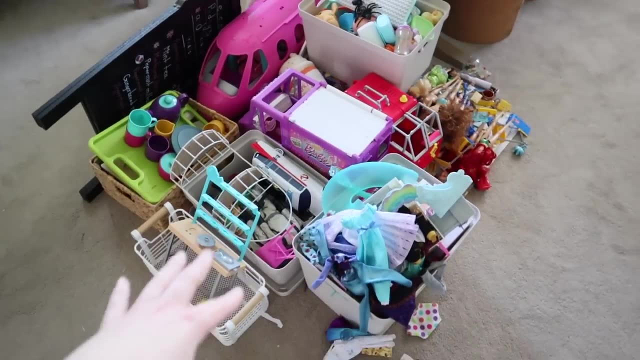 So I'm going to clean all this up, Get it where it needs to be, Bring in a box and like get this out of here so that the girls can't like try to sort through it when they get home, And then it'll be a nice clean playroom. 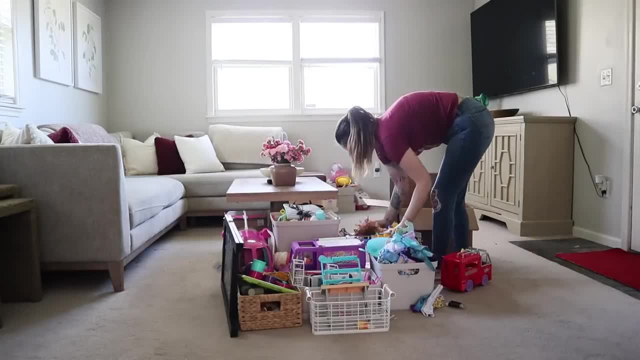 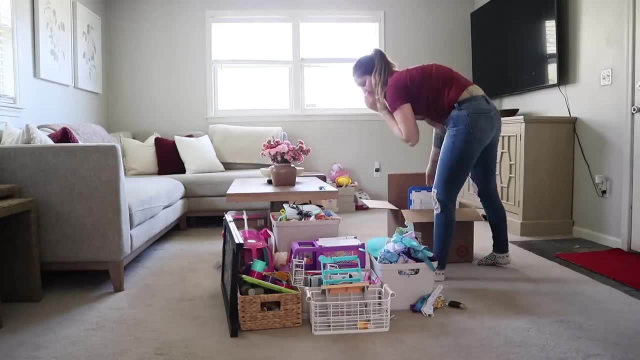 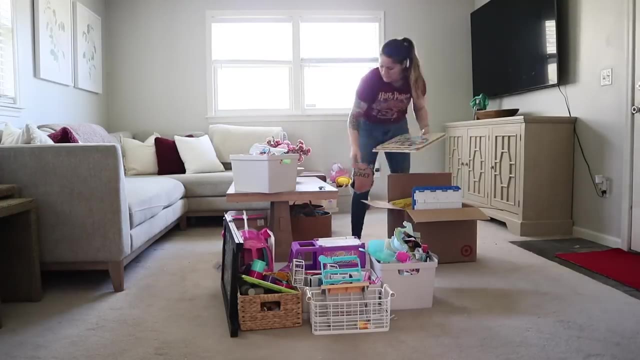 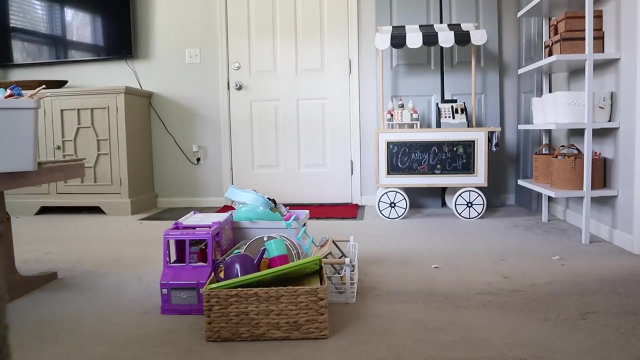 I can show you how everything turned out. I'm going to take my pytanie pique And then a lot of the autuelles are getting beaten like that. I'm going to go all up. I can watch the video and I'm going to go, and I'm going to go to theulk this. 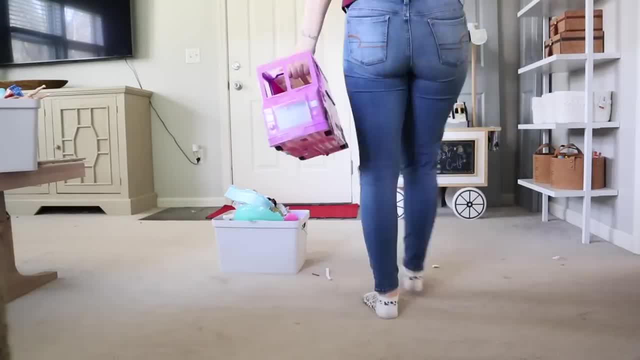 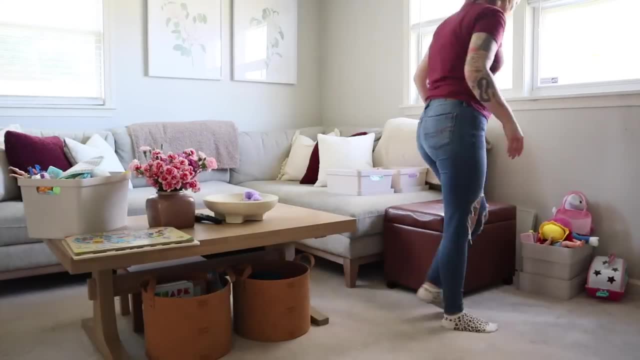 I cry. My mom turned off my main TV, and that's right. This one On Tuesday September 5th I couldn't film with So I was so confused. All I feel is useless Trying to fix a problem you can't admit you want to fix. 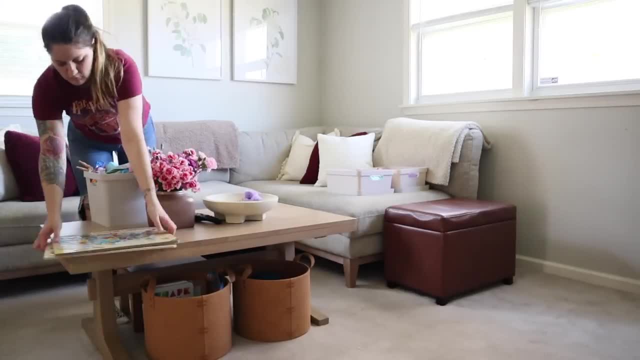 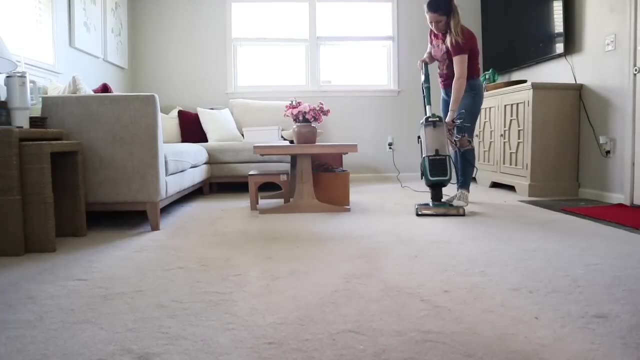 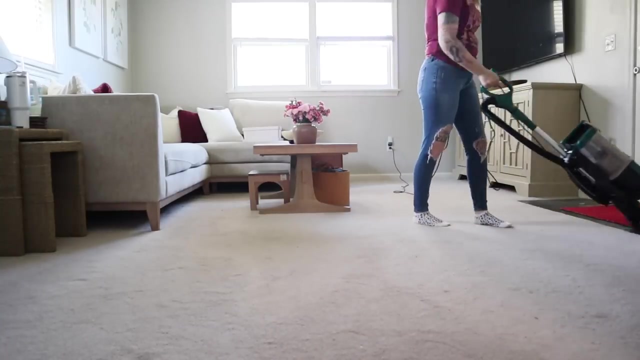 Why can't you be truthful? Honesty is crucial. Promise you that I'll be fine, baby. I can take a hint. You know Talking about stuff And You don't want to kiss, Holding hands or makeup. you say let's not. so i really, really wanna know what the hell you're waiting for. 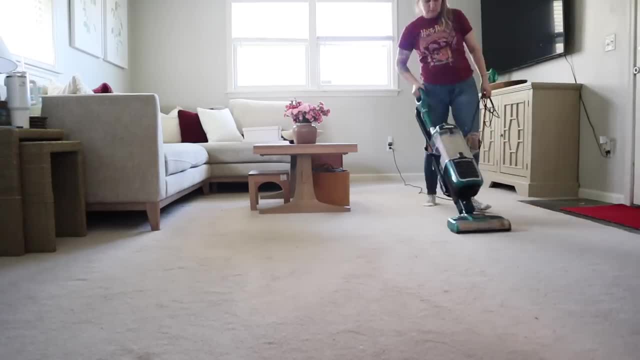 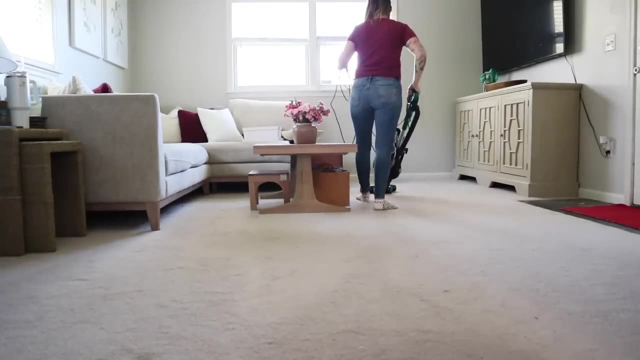 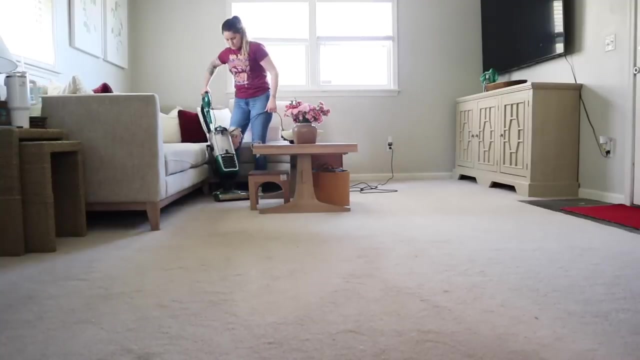 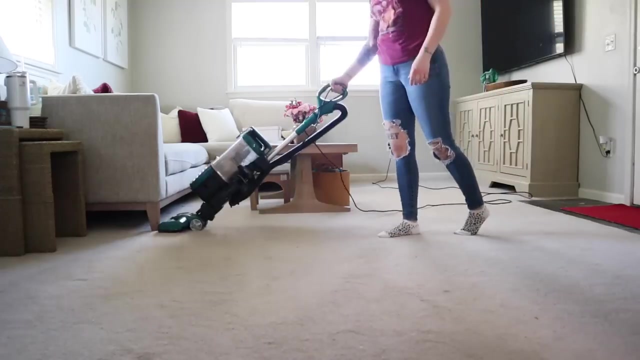 really, really wanna know what the hell you're waiting for. easy breezy. nobody said that love is easy, but you can go around pretending i'm yours when i'm not. oh, help me. help me, because i already have somebody else. she's in love with me, and the name is myself. this is so confusing. all i feel is useless trying to fix a problem. 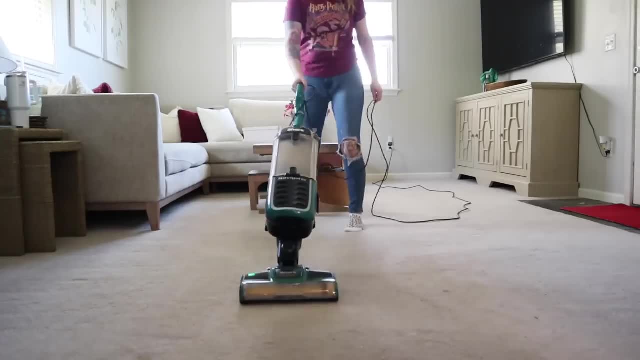 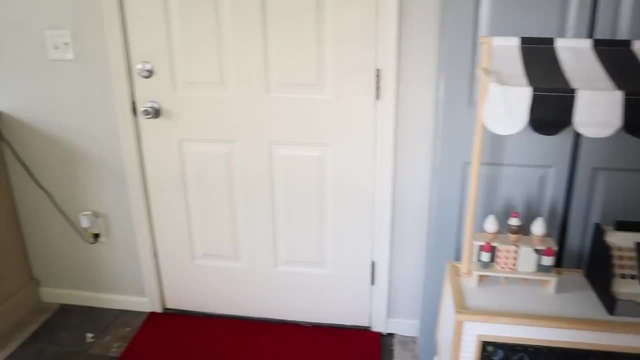 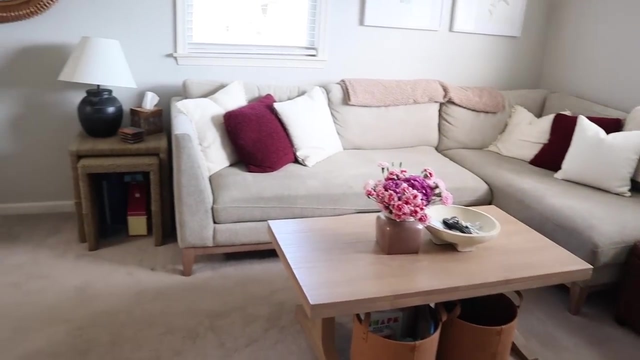 can't admit you wanna fix? why can't you be truthful? honesty is crucial. promise you that i'll be fine. okay, so it is the next day, and i just wanted to give you guys an update about how all the organization worked out what it's looking like now. the girls came home from school. 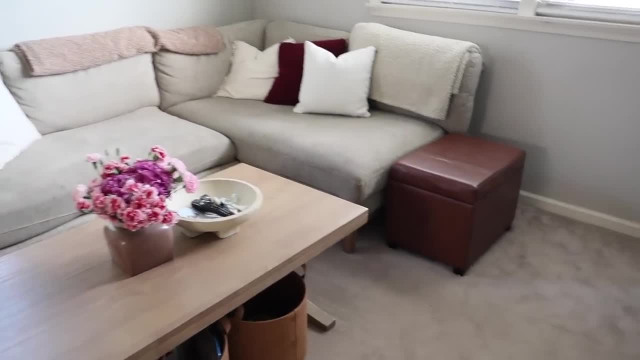 yesterday and i just wanted to give you guys an update about how all the organization worked out yesterday. and i just wanted to give you guys an update about how all the organization worked out, saw everything they did- play with their toys, put them away- so we have an idea of how it's. 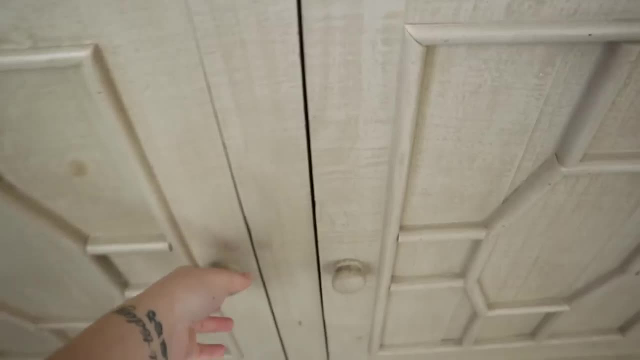 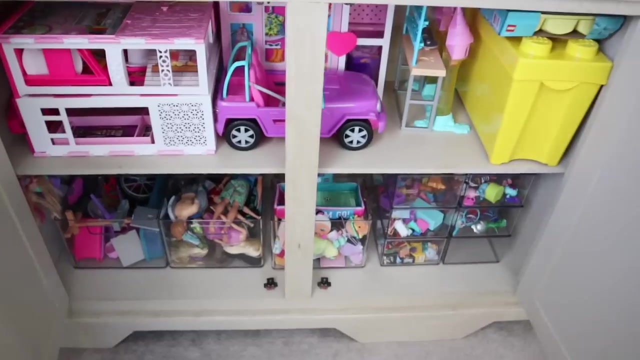 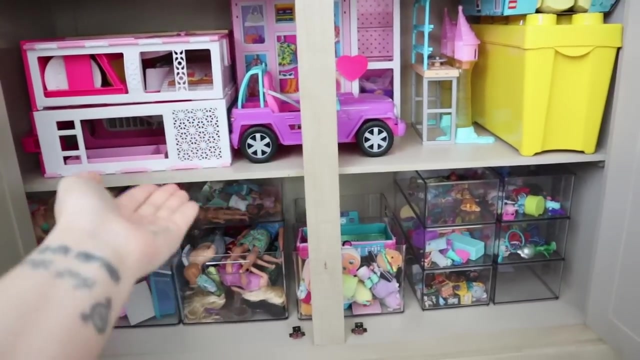 functioning and a few things changed, so I just wanted to show you what we ended up with. I think this media console is my absolute favorite. I decided to keep all of their pretend play toys in this larger section because clearly they do have so many- all of the larger toys and accessories. 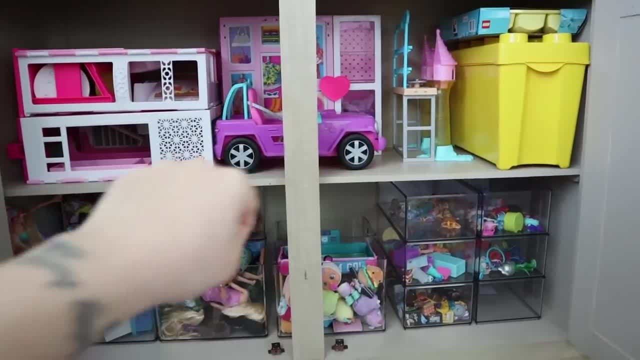 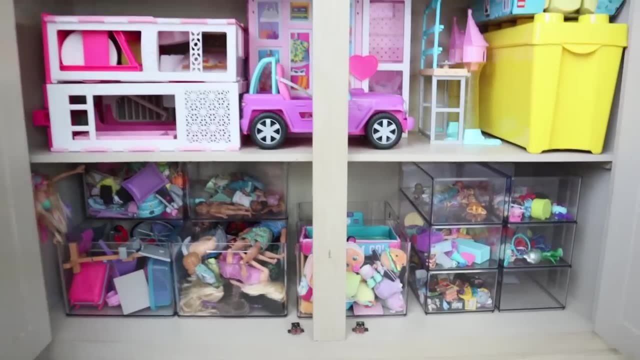 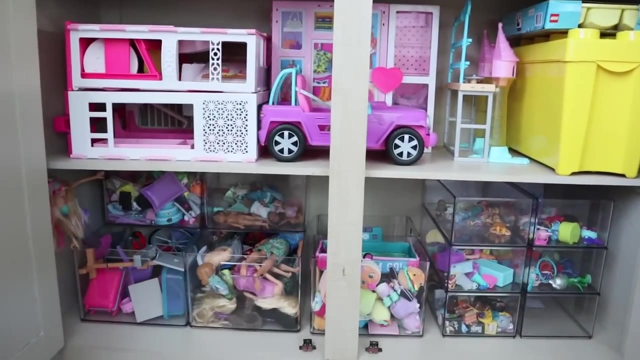 up on the top, so like their Barbie houses, Legos, things like that, and then we put all of the acrylic bins on the bottom, so all other toys, and I did still kind of section it off. like you can see, Barbie is right here and then there's like other toys right there, but the girls loved this. 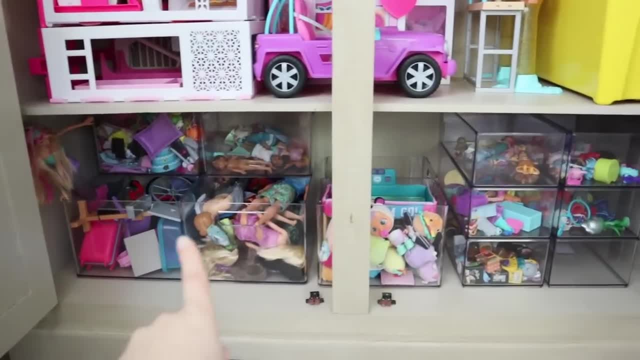 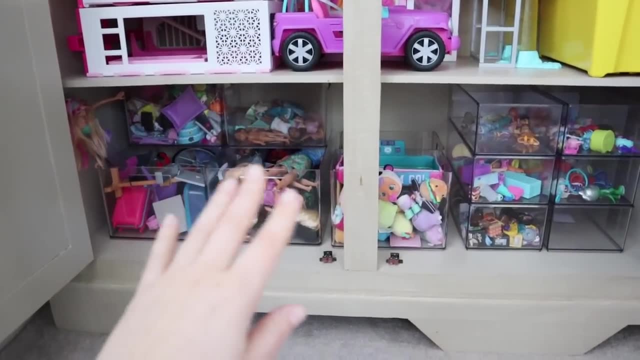 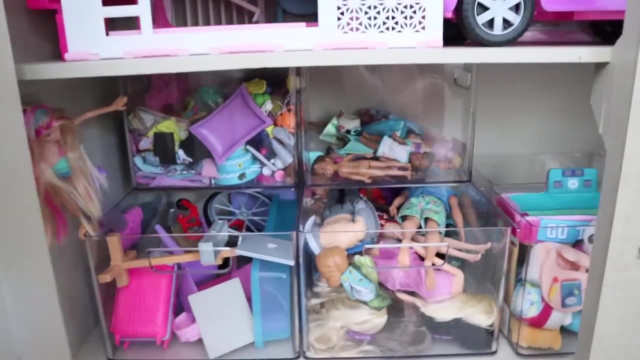 of everything they saw yesterday, everything they played with these bins. they couldn't stop thanking me for doing this, which made me feel so good and so bad at the same time, because it's like what took me so long to address this issue for them, but these ended up working out so well. so I have two of these larger bins down here for the larger Barbies. 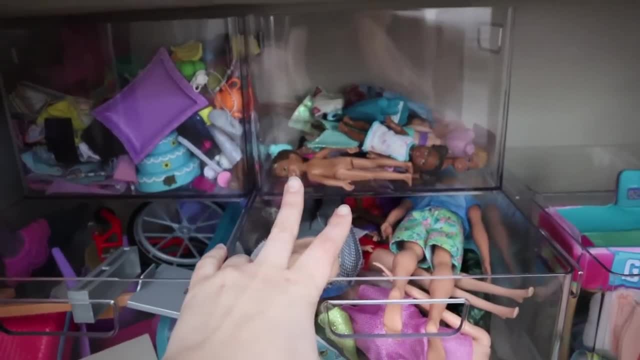 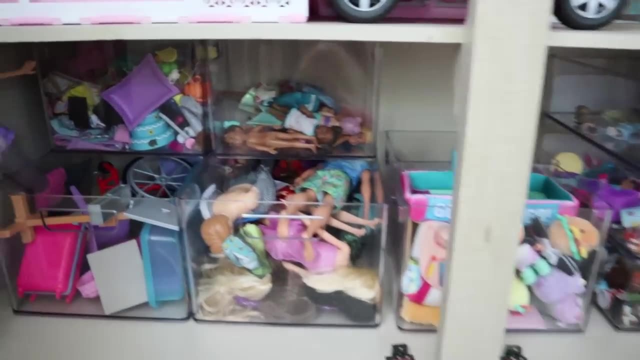 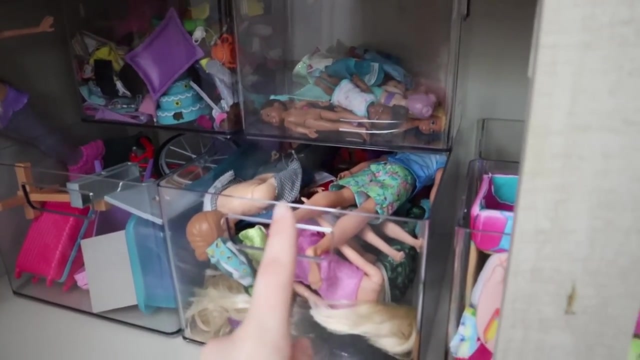 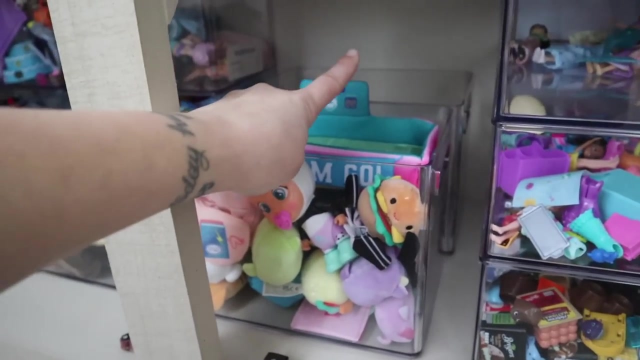 larger accessories and then some stocking half-size bins on top of them for, like the little kid, Barbies and tiny accessories. that worked out like better than I could have expected. they love it and they have no problem putting them back and stacking them, so it's just worked out really well. I have all of Sawyer's little mini squishmallows in here and 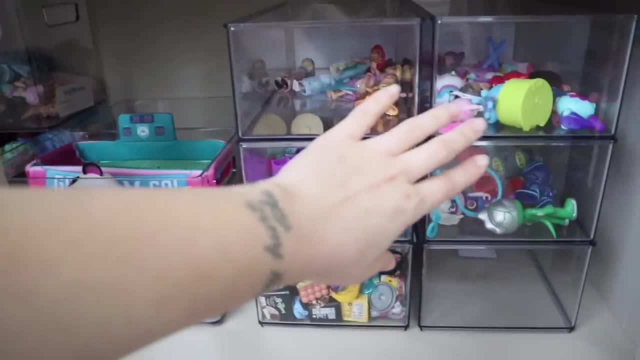 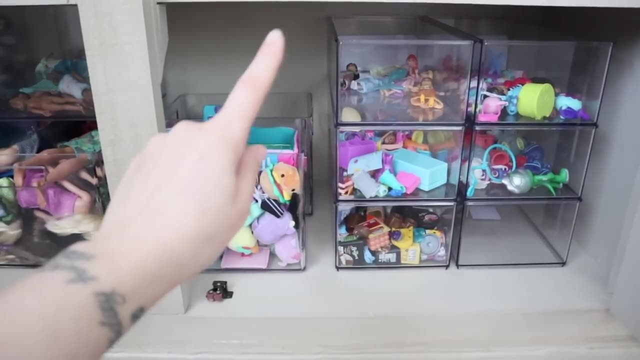 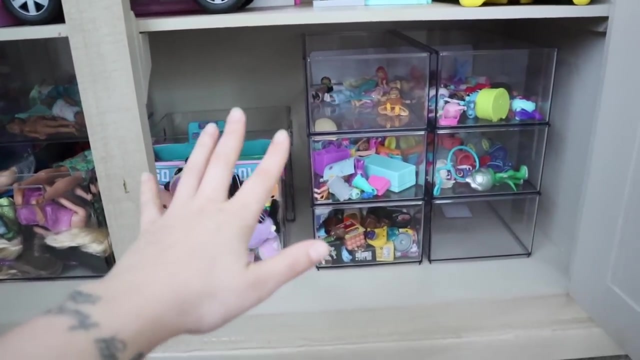 then there's an empty bin in the back and then all of these are like tiny toy play sets with an empty bin down here, and that's also like number one piece of advice: make sure that you have room to grow in whatever organization system you're trying to implement. if you don't, it will. 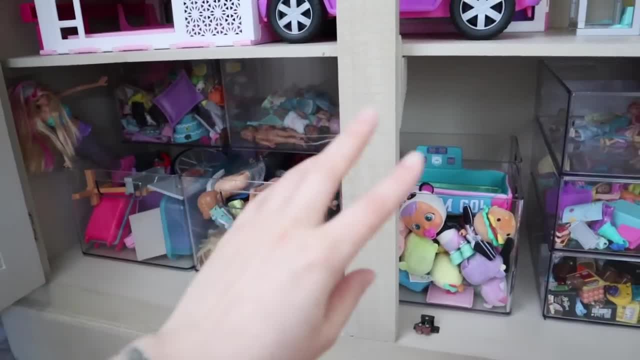 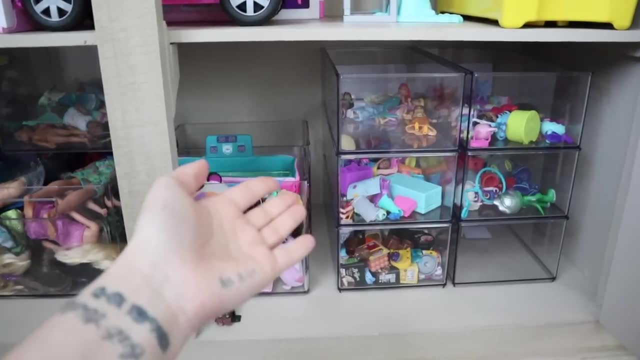 fail, unless you're following the one in, one out rule. but if I didn't do that, have some empty bins, then as soon as we bring anything else into this space, there wouldn't be a place for it. but anyway, all the pretend toys are on this side, and then all of the 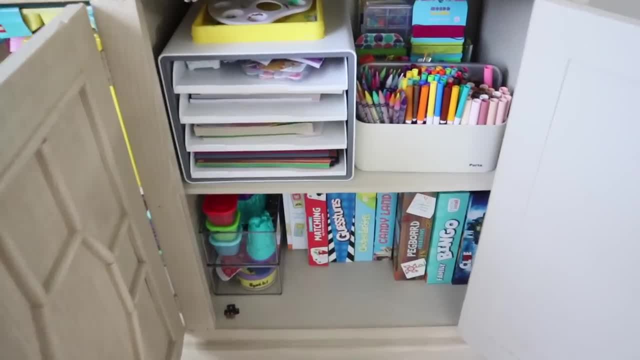 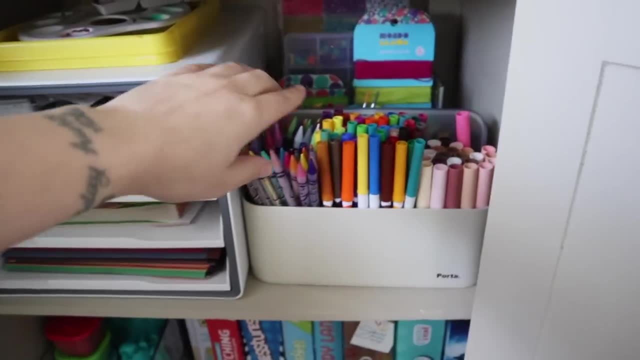 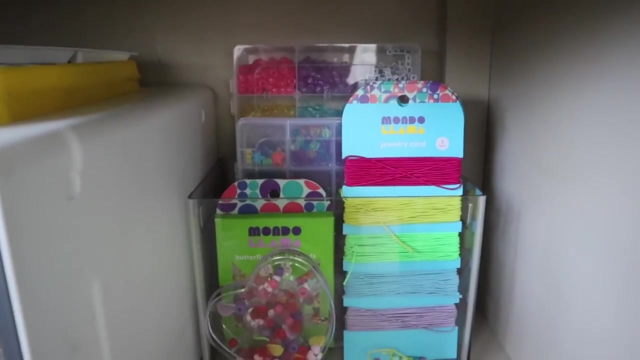 crafts and games. I did keep over here and I'm glad that I did, because it worked out really well. so all the craft things, art supplies, are still on the top, and I think I talked about this but didn't show it. I did add in: the girls have all of these, like beads and jewelry. 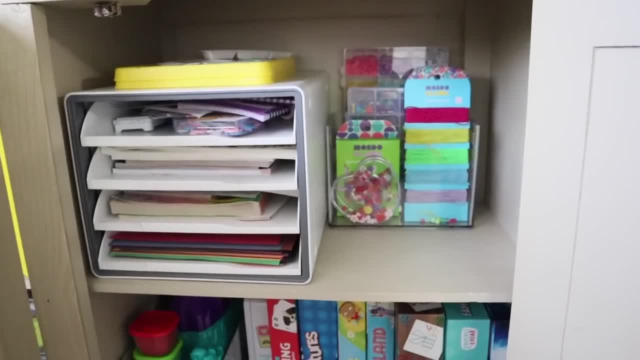 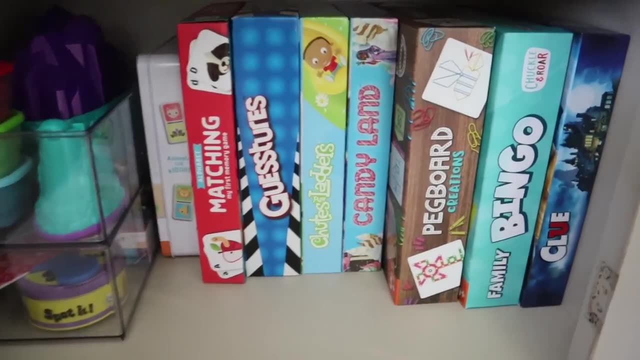 making accessories. so I just had Derek go to Target and grab another acrylic bin for me and it worked out really well to keep that and then down here with their board games. I did make a small change, so I like that. all of the games are upright. like this. you can clearly see which. 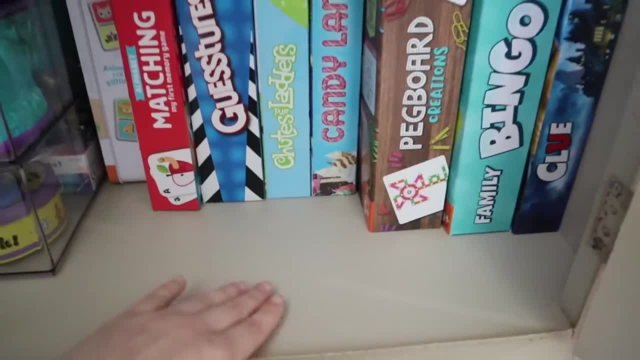 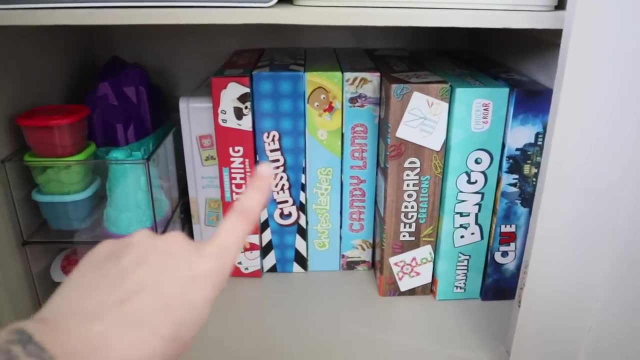 ones they are, and just pull it out and then put it back in. I previously had them stacked going this way and you'd have to either pull a bunch out or it would just make a mess. so I feel like this is going to work a lot better. it's like books on a bookshelf, and then I changed over. 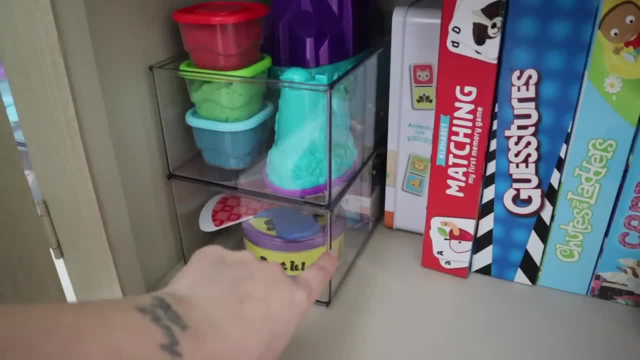 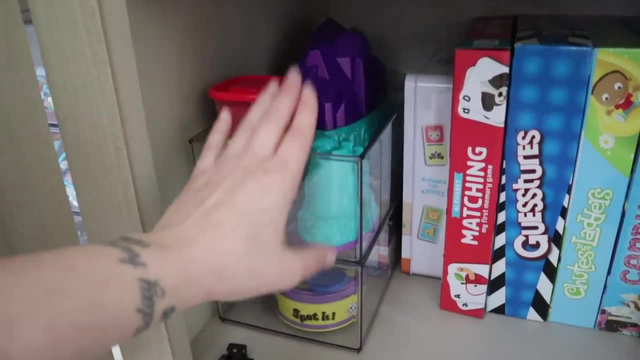 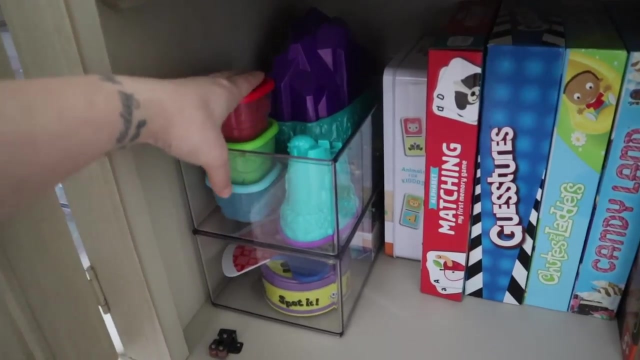 here. I did have just one deeper acrylic bin for all of those card games and things, but I ended up with these stacking ones so that we still have the card games. and then I put Sawyer's kinetic sand up here. she is loving that her kinetic sand has a home now. typically we just like. 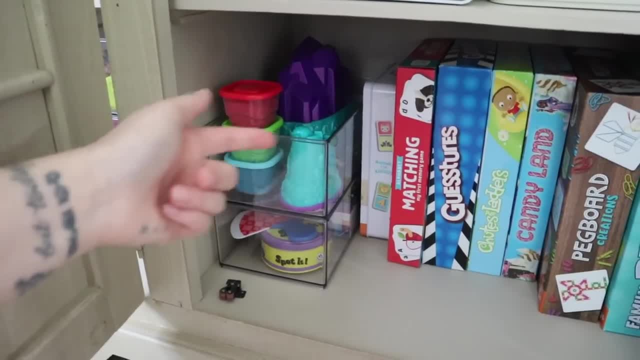 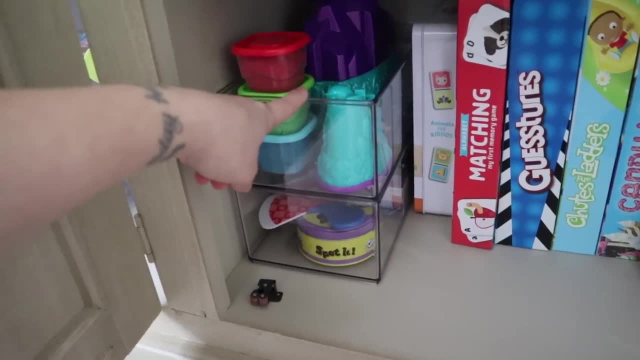 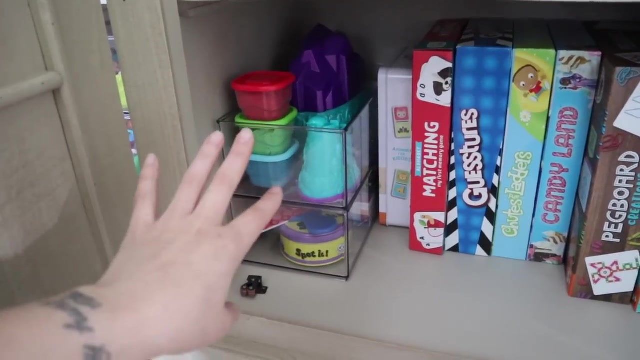 leave it around. it's either on our laundry folding table, on our kitchen table, something like that. now there's a designated space. she is appreciating it so much and she said to me that she loves it's in a bin because she could dump it out in the bin and make her own sensory bin, which is like so cool that she's even thinking of that. 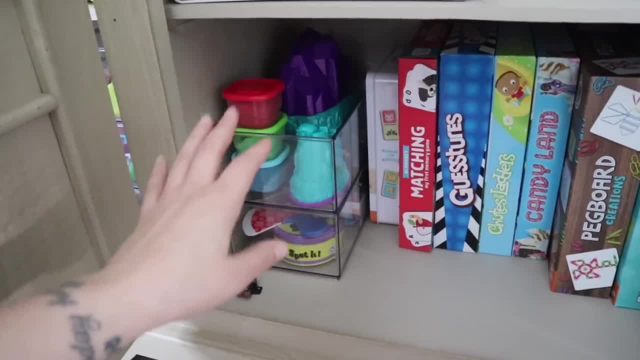 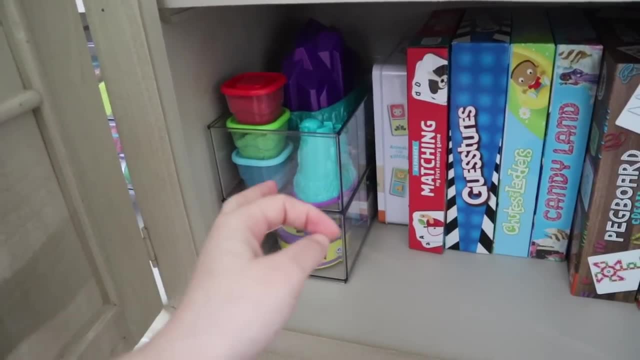 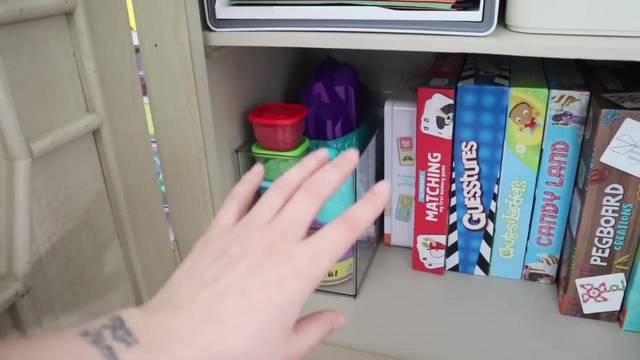 and before anybody freaks out. we are very blessed that our kids can play with like Pleidow, slime, kinetic sand very responsibly. we've never had a mishap with any of those items, so we feel fully confident in letting her have complete and full access to it. if something does happen, we'll have. 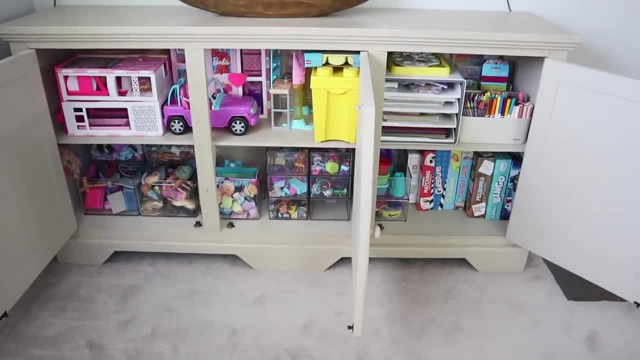 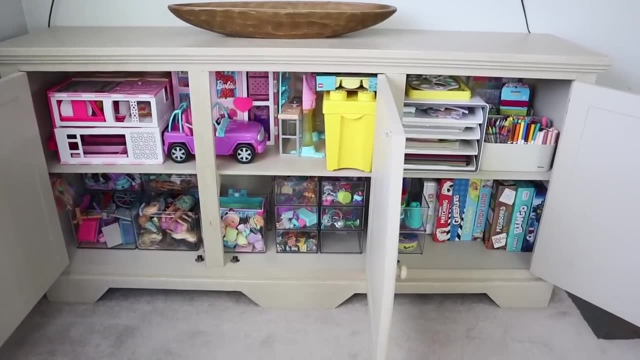 change that, but I just don't foresee it being an issue. So this is definitely the most well organized this media console has ever looked, and the girls were playing with all of these things yesterday. Loved them, Had no problem pulling anything out or putting anything away, so that's. 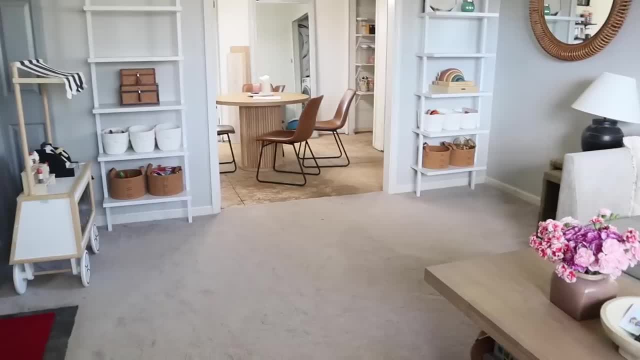 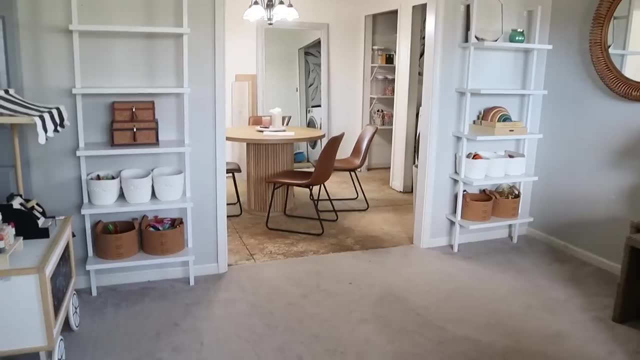 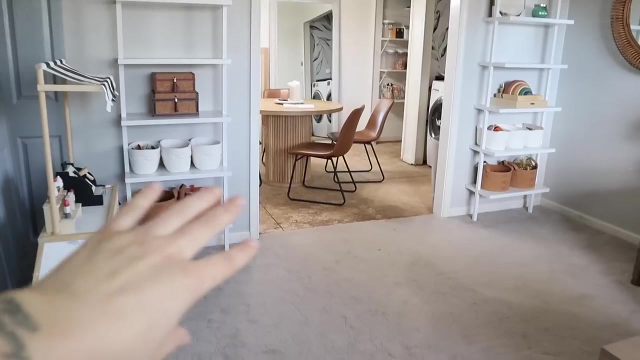 an A plus, in my opinion. I'm loving this system so far. On the other side of the room, we do have these two ladder shelves that like frame the doorway, and we like to use the lowest rungs for additional toy storage, just because our kids can easily reach that. Both of them can, and this is a 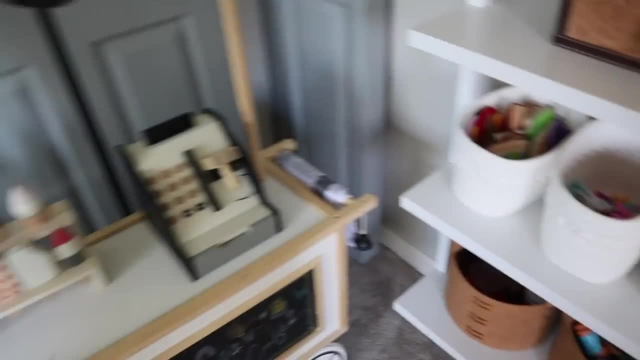 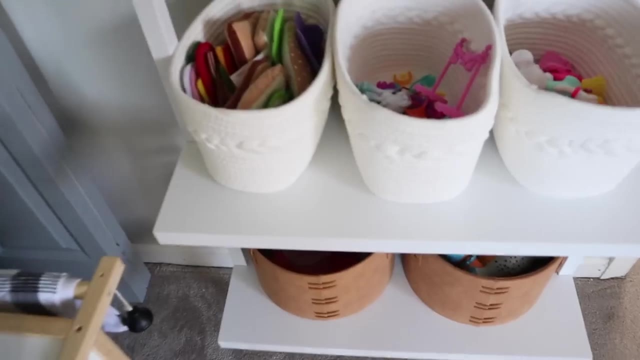 playroom, so everything can't be purely decorative. This is the girls market cart. They love it, especially when they have friends over. This is like the most played with toy and next to it I just have this little bin of felt food for like a sub shop play type of scenario. 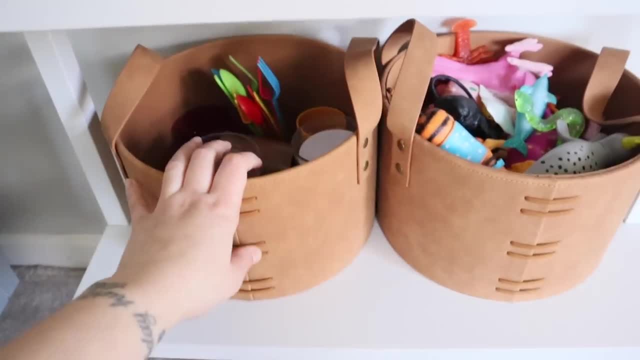 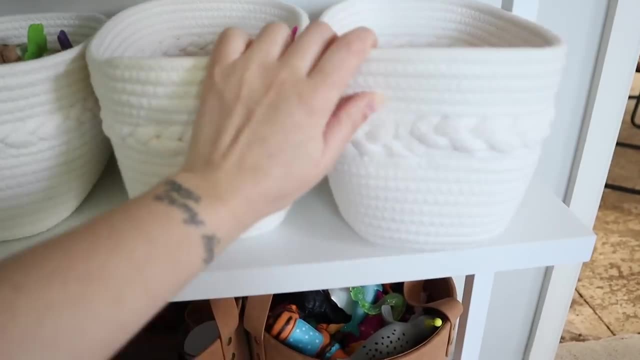 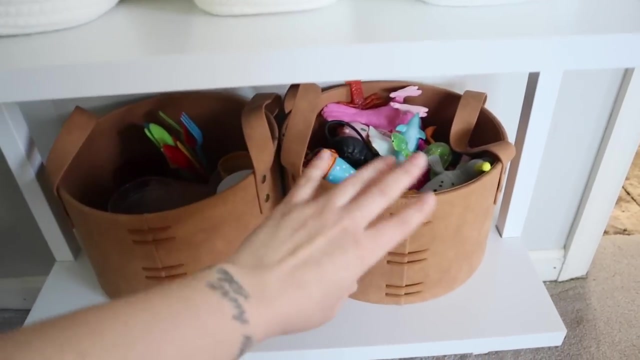 And then these are plates and drinks and silverware, so those go with the market cart and then next to it. I also use these extra two for some tiny toy play sets and Sawyer's party animals. Those are like the love of her life. She loves these so much so I like to keep them out and 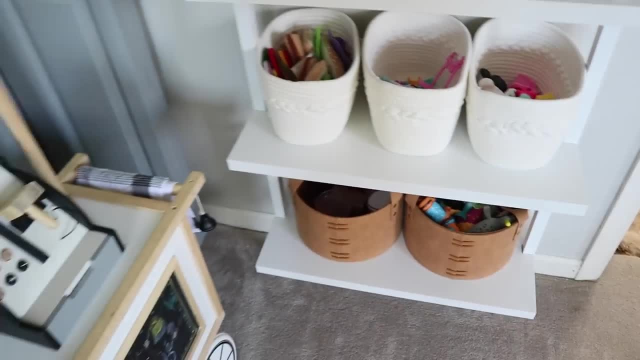 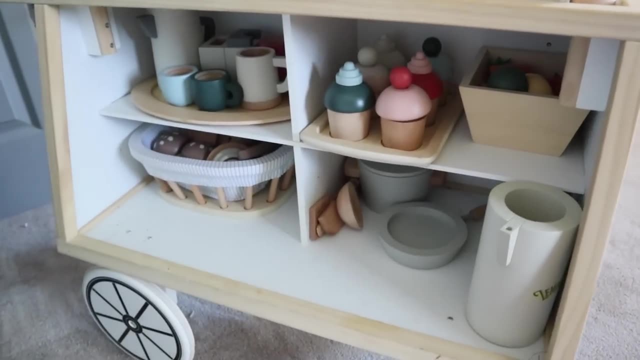 accessible at all times. Easy cleanup- That's what we've got going on over here. and then the market cart is currently set up for an ice cream stand, but on the other side we decluttered at least half of the food sets that were in here, Simplified it quite a bit. We've got their bakery. 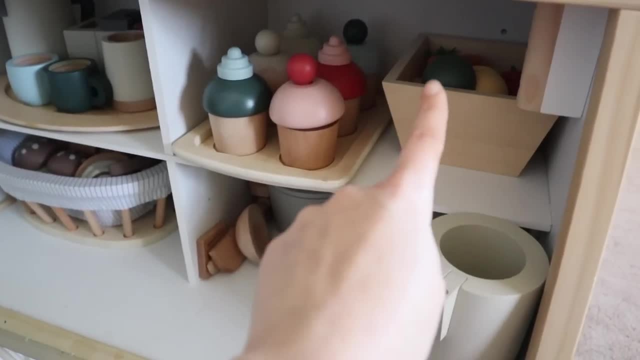 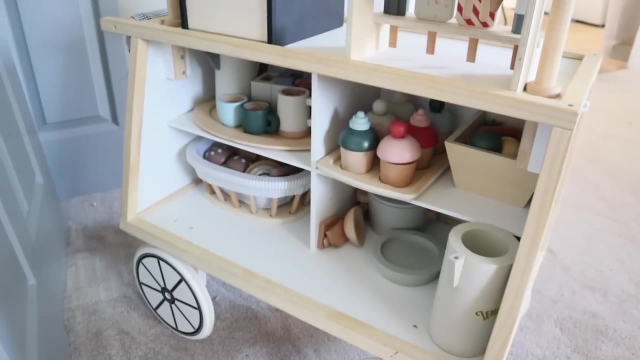 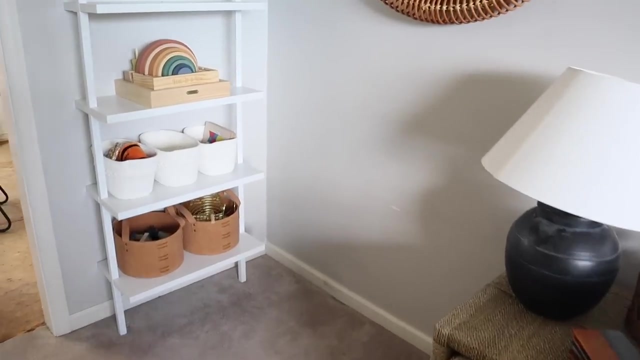 set, cocoa set, cupcake set, fresh produce, lemonade and cooking utensils, pots and pans, things like that, and now it all fits in there really well, They can see it and they can set up like play scenarios a lot easier. And then over on this shelf we do have some more board games that are just like pretty. 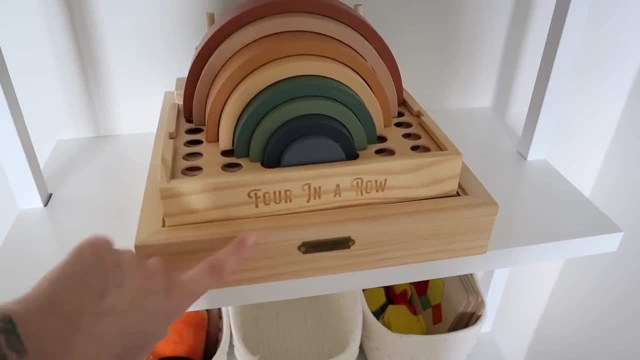 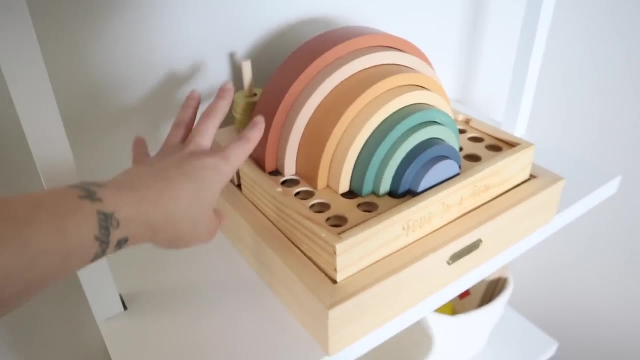 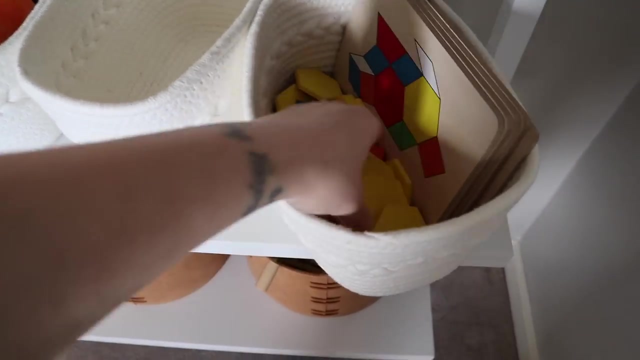 so I keep them out As decor as well. but this is a chess and checker set, This is connect four and then like a rainbow stacker and this is a little like math activity for Sawyer. So we have this here and kind of going along with that same theme, is these like shape boards? I don't know exactly what they're called. 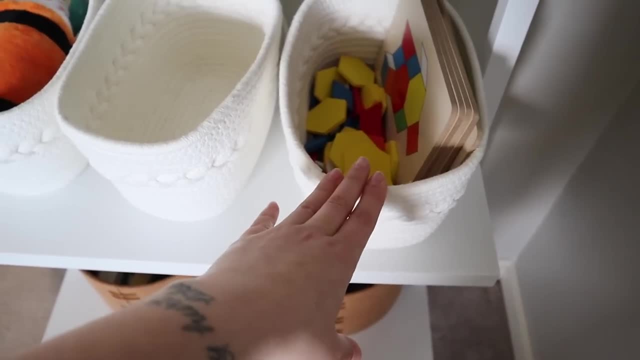 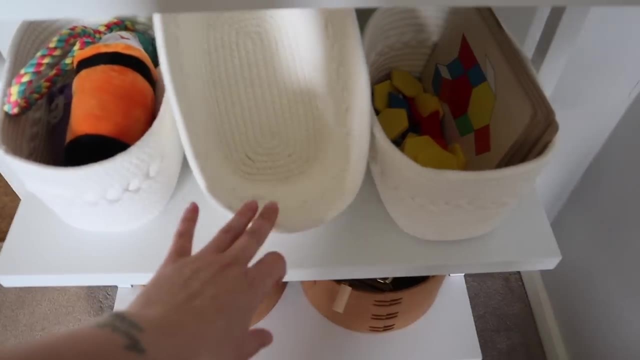 but I remember playing with these when I was a kid, so it's crazy to me that those kinds of activities are still around. And then dog toys and an empty bin again for growth. I cannot stress it enough. That is so important to make sure you have room to grow Down. here we have wooden blocks. 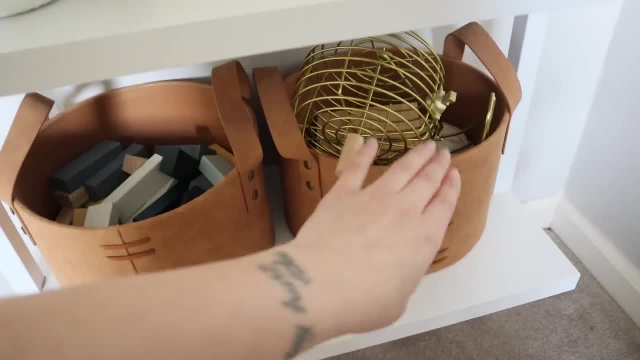 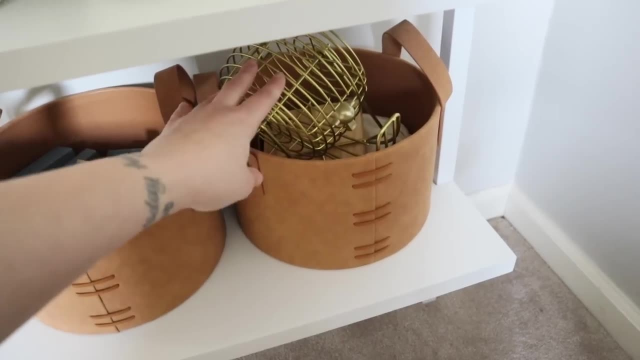 Jenga and a really nice bingo set. We love this thing, but it has been hard trying to figure out how to store it. Even in this storage container it's still peeking out, but it's okay, I'm trying not to let it. 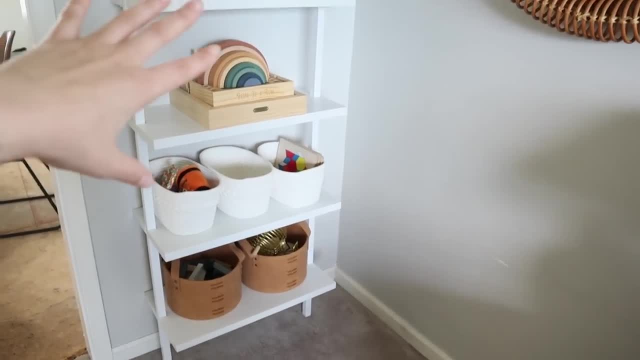 bother me, That's just like an OCD thing, but other than that, we've got all of this straightened up Room up here for some decor. I'm going to be decorating this weekend and I've been really excited to be here since the beginning of the semester and I've been excited to be here since the beginning of the. 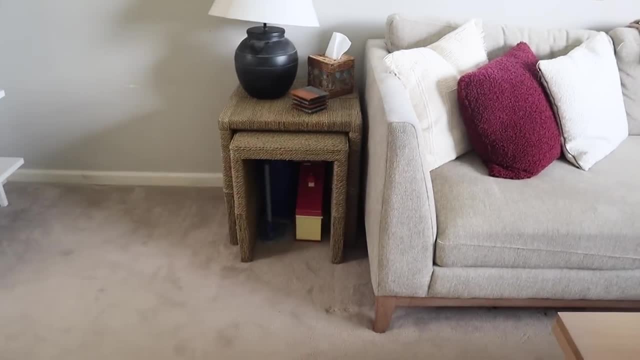 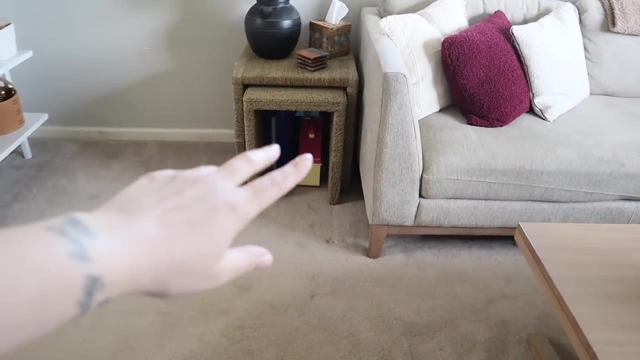 so look out for that video. and then, if you remember, over here all of those Barbie houses and things were just spilling out. Sawyer, bless her heart, she's so cute. but she was trying to clean up one day, didn't know where to put them and so she just like stacked them out here. so 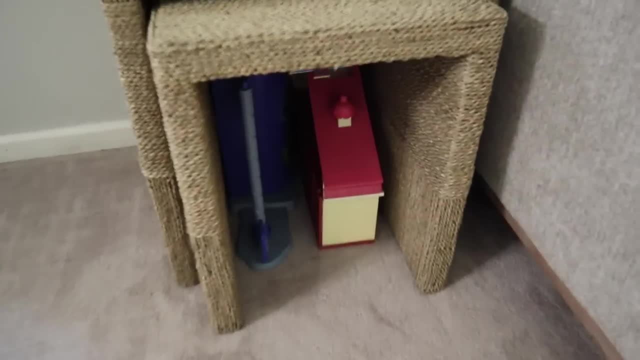 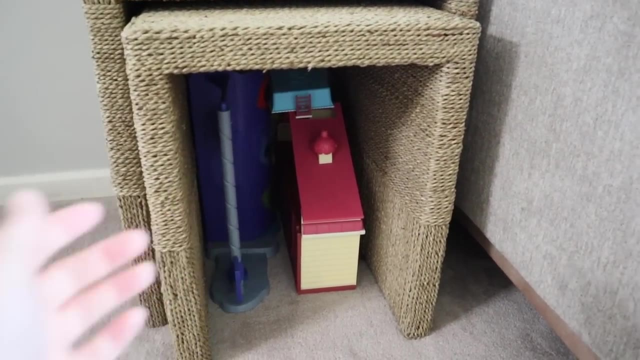 we have the Barbie shelf now, but in here I still have some hidden storage. we've got the girls bluey house and all the characters fit into there, and then the PJ mask HQ. we try to find new and inventive ways to like store toys because they've clearly overtaken our house. so we've got a couple.